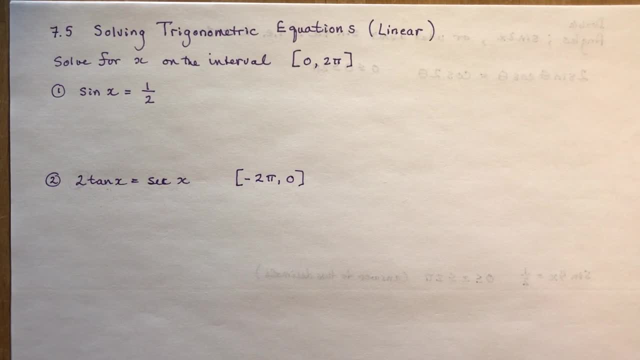 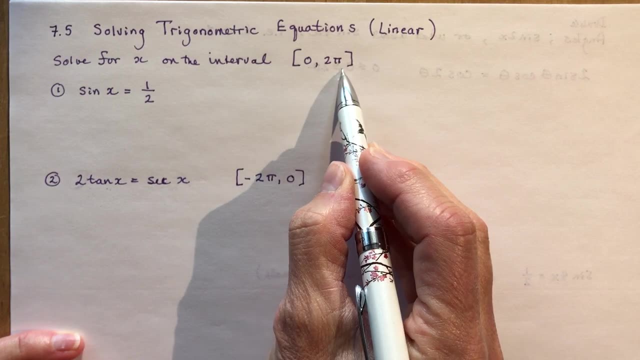 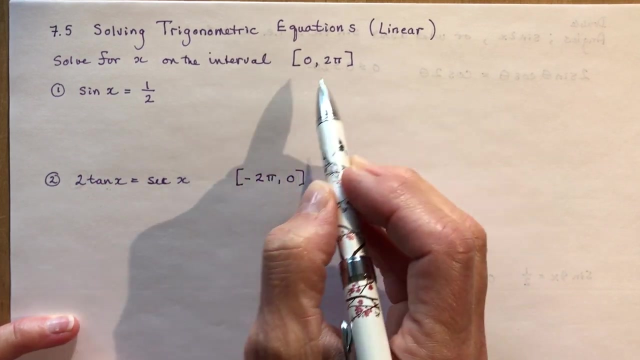 stretch or compression. So we're going to start with this question here. sine x equals to one half. Now you will always be given an interval because, as you know, sinusoidal functions continue on and on forever and ever. so you would have an infinite number of solutions. 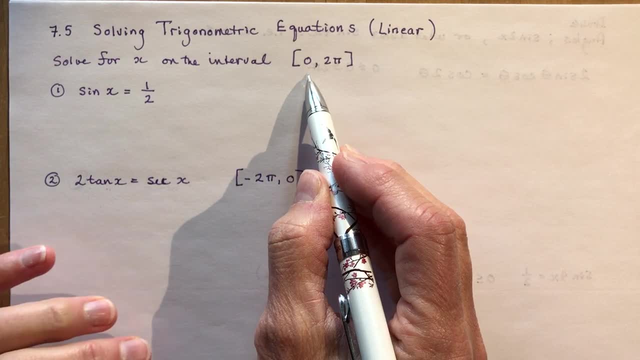 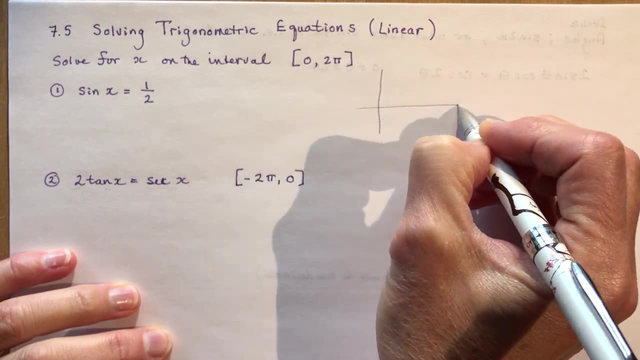 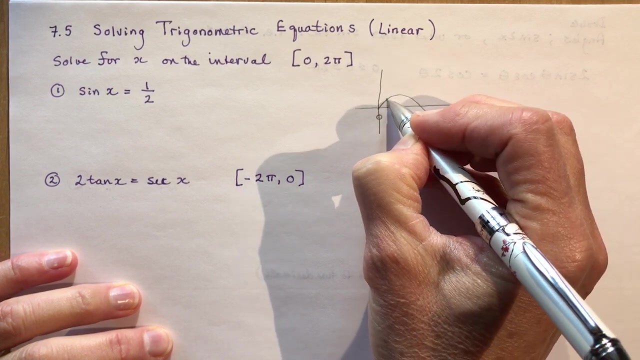 Without domain restriction. So where is sine x equal to a half? This should be second nature to you now, like breathing out and breathing in. So here we go. here's a sine function over the domain zero to two pi. Where is it equal to a half? So you know, the max is one, so it will be equal to a. 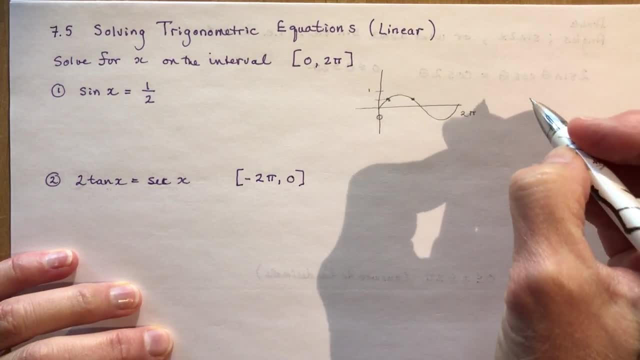 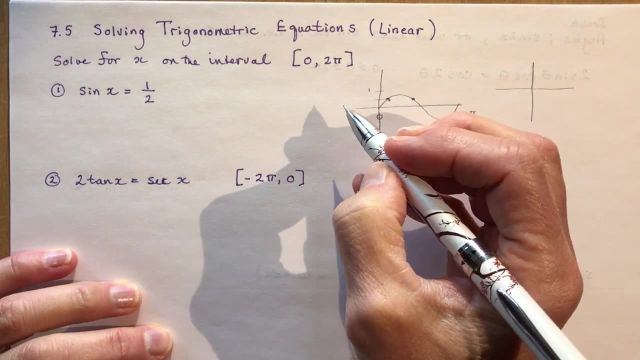 half in two places. Now that is not news to you, because you're also familiar with using cast rules to find the height of the water at, say, three o'clock, and you're also familiar with using angles. So you may be asked to find an exact value. If it doesn't say exact, I would give exact if it's. 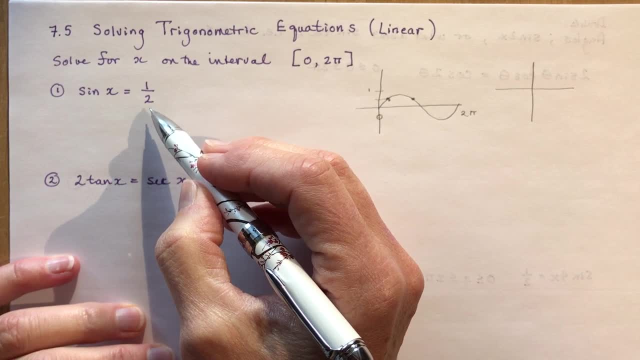 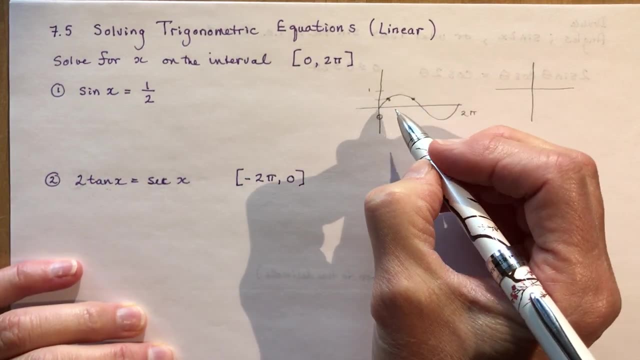 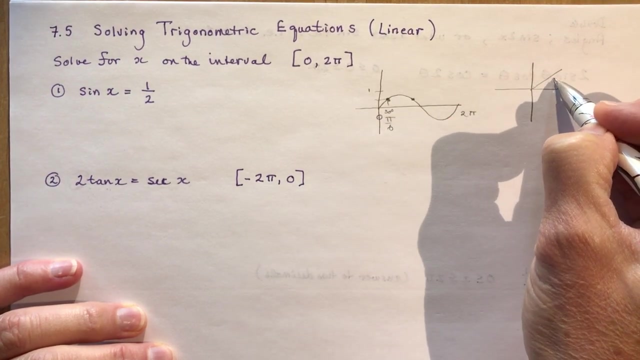 possible, For instance, a sine sine x equal to a half. You know that sine x is a half when x is pi over six or 30 degrees. So this would be 30 degrees right here, Doesn't that look like it? Or pi over six. So we have one solution here: pi over six. That's a pretty big pi over six angle. 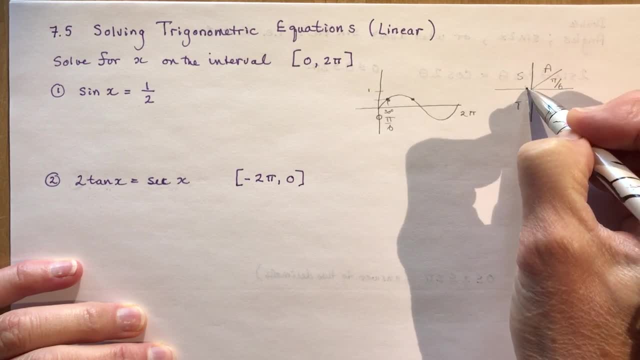 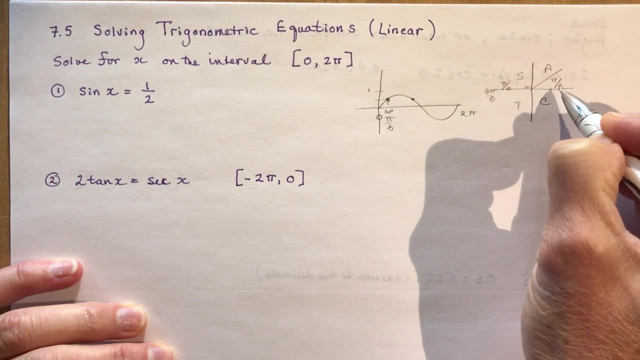 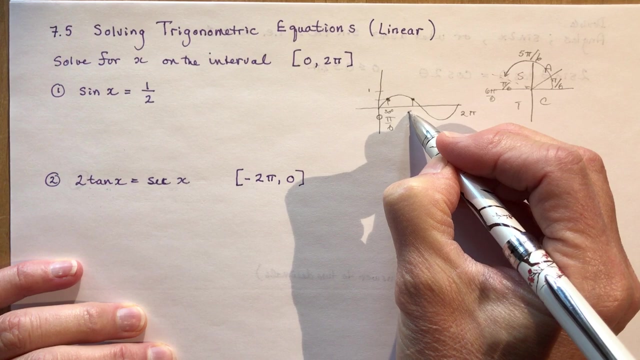 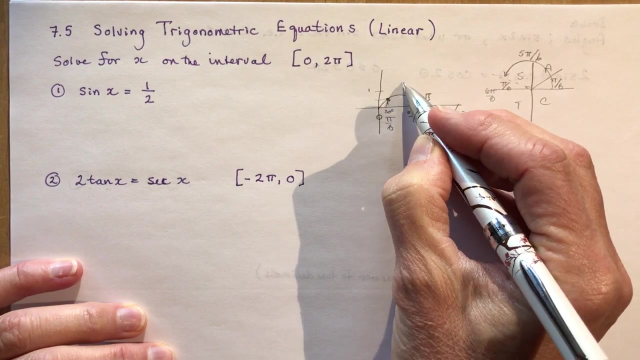 So that's my ACAST, And we have another one over here which would be pi over six, away from six pi over six or five pi over six. Okay, so that's this. one here is five pi over six. That also makes sense because this is pi here, And so, as you can see, this is my first quadrant. the second quadrant, the 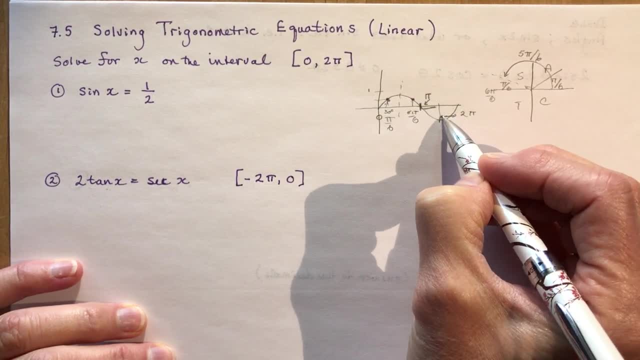 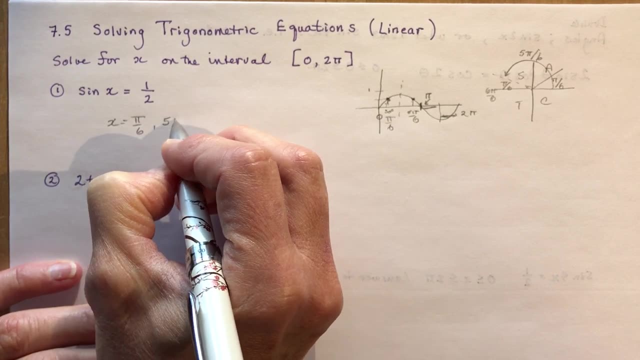 third quadrant, the fourth quadrant and this second quadrant. So you can see that this is an goes from here to here and the fourth quadrant from here to here. so that means x is going to be equal to pi over 6 and 5 pi over 6. okay, that's just to warm you up. let's do one. that's a little. 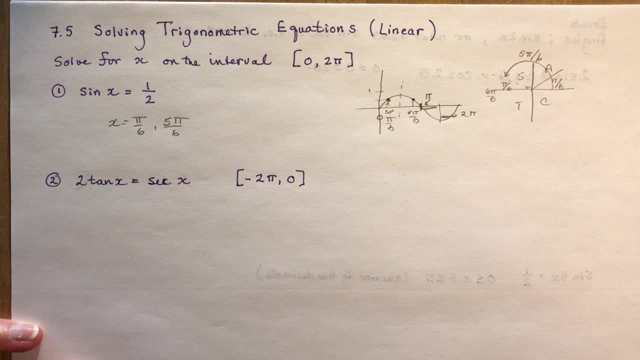 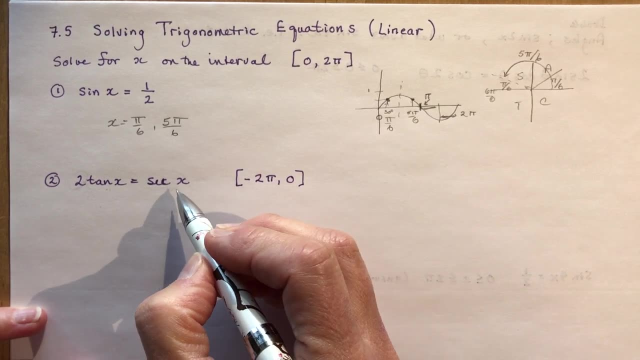 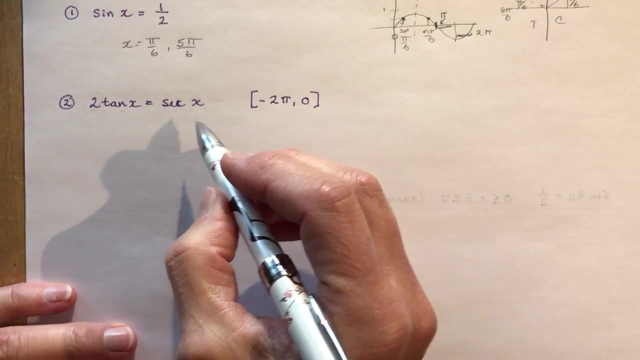 more difficult now. so this one we have, 2 tan x is equal to secant x. so when you're working with these equations, what you want to do is to move things to the other side of the equation, because what you want to have here is: you want to have a number on this side. okay, you don't want something. 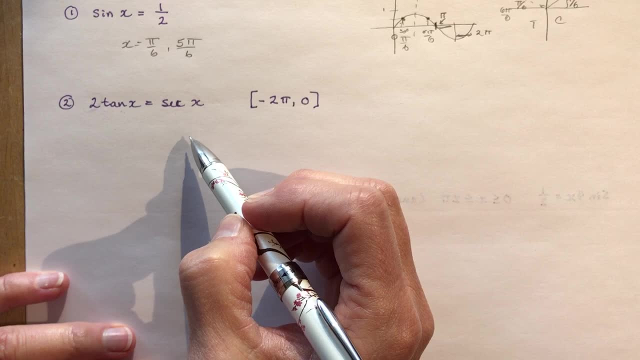 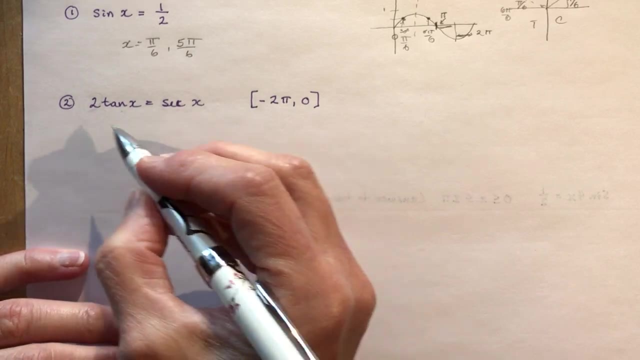 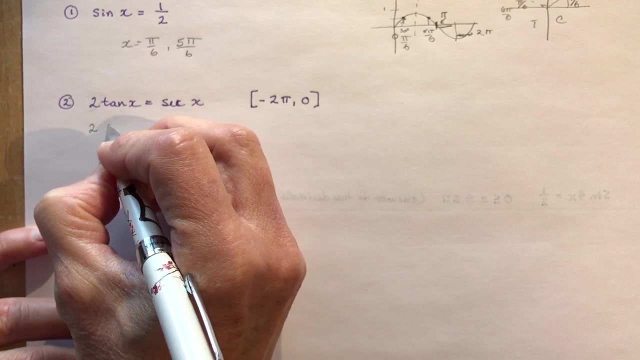 equals to another function and you want to, really, if you can get it down to one function. sometimes that's not just possible. so let's see what we would have if we wrote 2 tan x and we're going to use an identity, which is that tan x is equal to secant x, and we're going to use an. 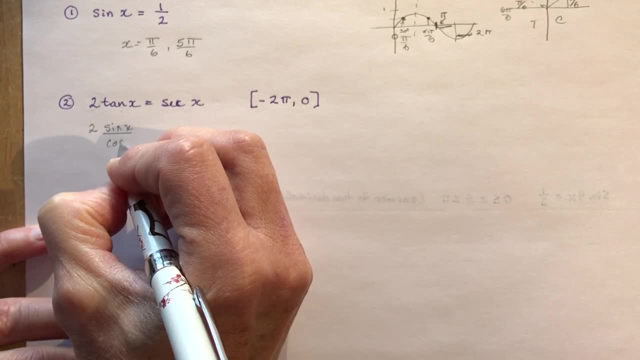 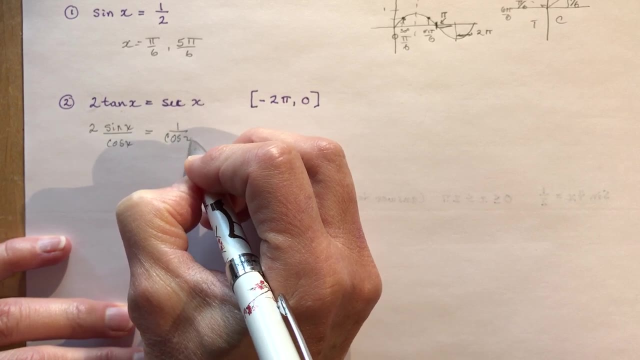 identity which is that secant x is equal to secant x, and we're going to use an identity which is that equal to sine x over cos x, and secant x, of course, is 1 over cos x. So if I bring this to the other, 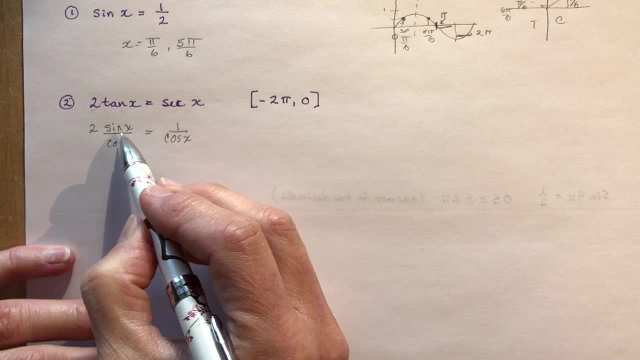 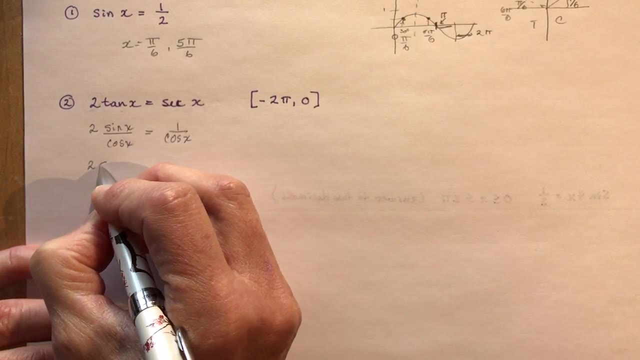 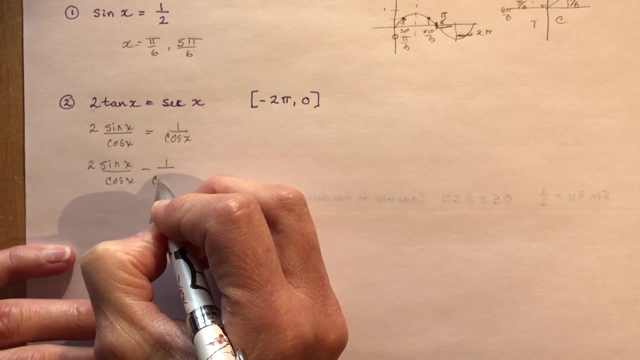 side of the equation. I can have an equation that has a numerator that I can solve for. So if I bring this over here, I know it all looks like magic, but once you've done a few you'll say, oh yeah, that's what I should do. I should just move that over there. cos x like that right. So I moved it to the 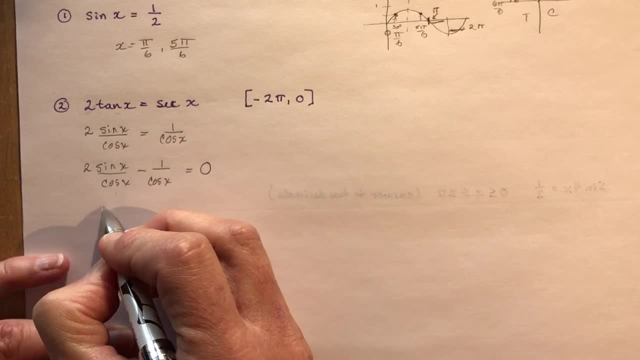 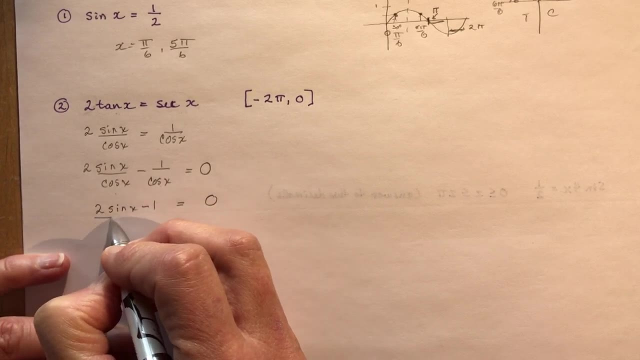 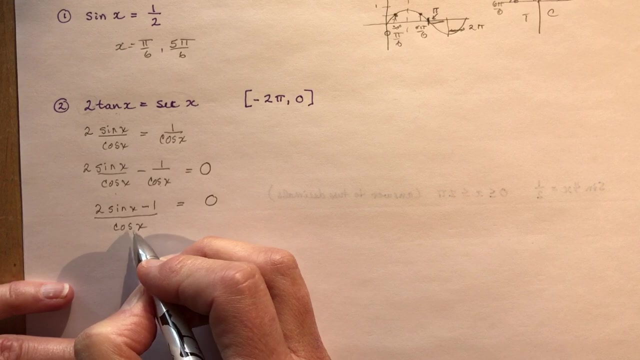 other side and because the denominator is the same, that's the same as me writing: 2 sine x minus 1 is equal to 0, still over cos x. but this becomes unimportant when I'm solving an equation because, as you know, the only way this could be equal to 0. 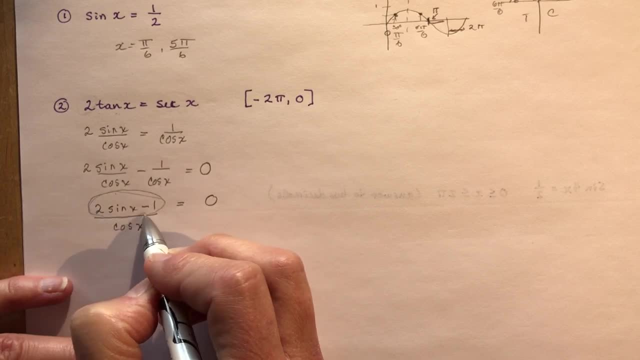 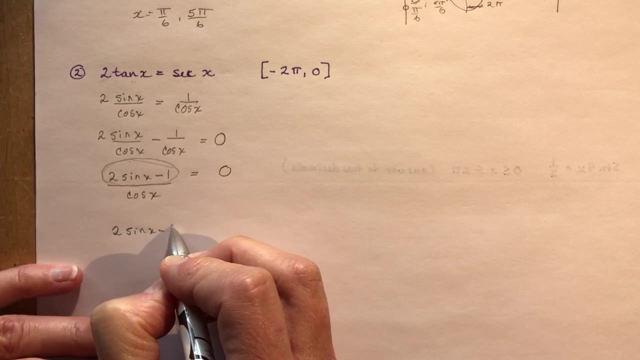 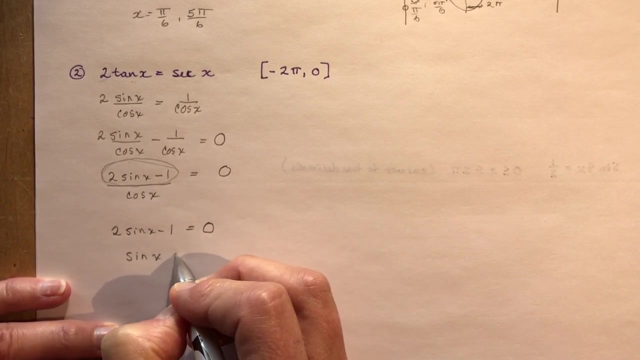 is if the numerator is equal to 0. So that means all I have to do is solve 2. sine x minus 1 is equal to 0, and now I'm going to throw everything back to the other side of the equation, so I just have: sine x equals one. 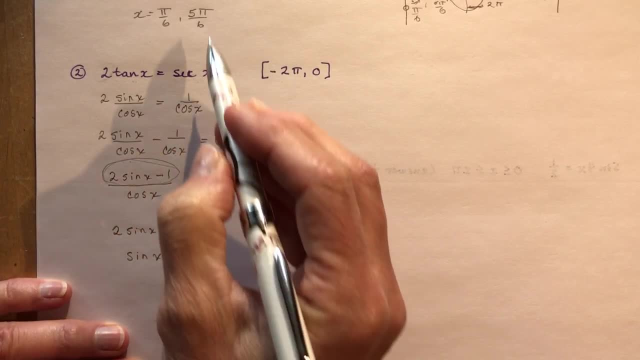 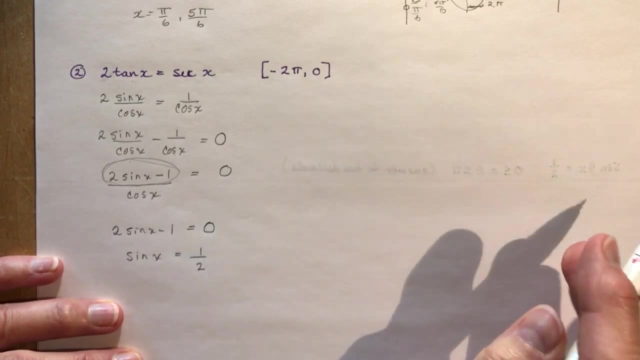 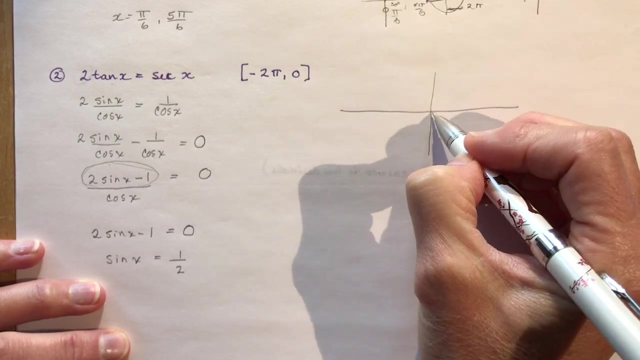 half. Okay, so I'm back to the same question we had above, except the domain this time is between minus 2 pi and 0.. So if we- well, maybe I'll draw it again here- so if I have sine x, so it's going this way for 2 pi and it's going this way to minus 2 pi. 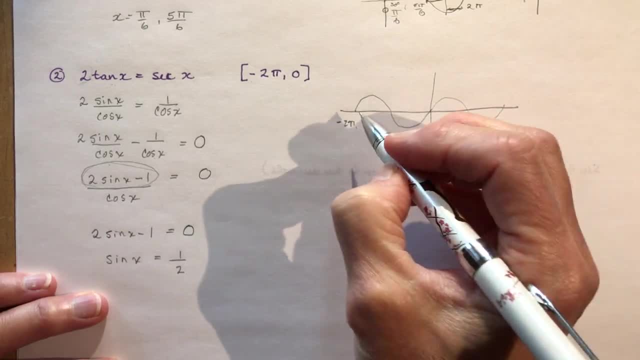 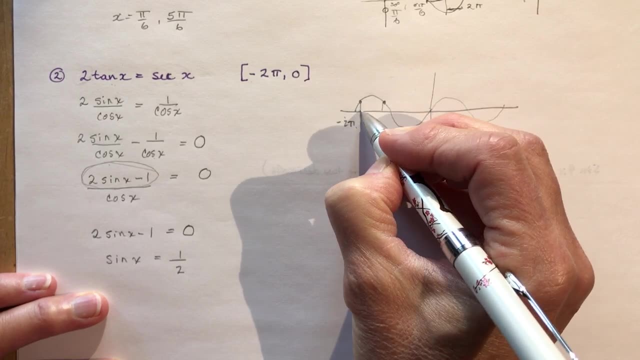 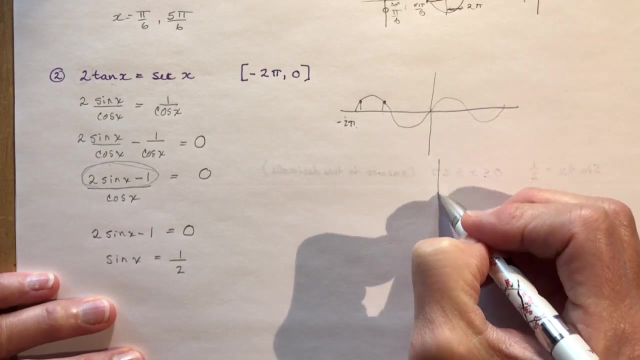 So I want to know where is sine x between minus 2 pi and 0? so in this domain here, where is it equal to a half? and I'm trying to find these two spots here. So you do know that if you're doing negative angles, 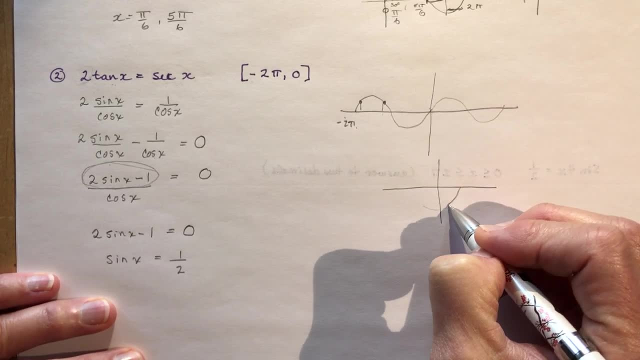 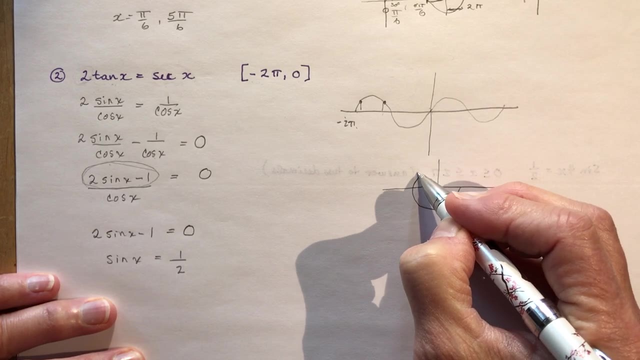 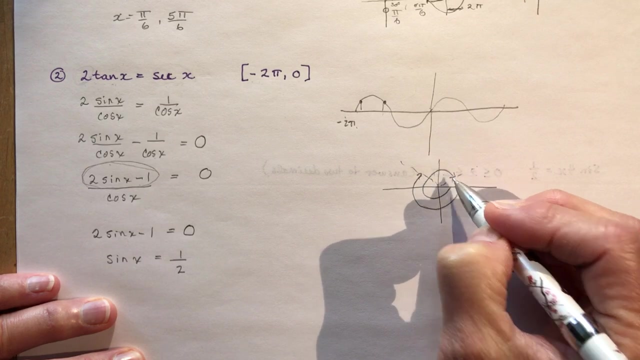 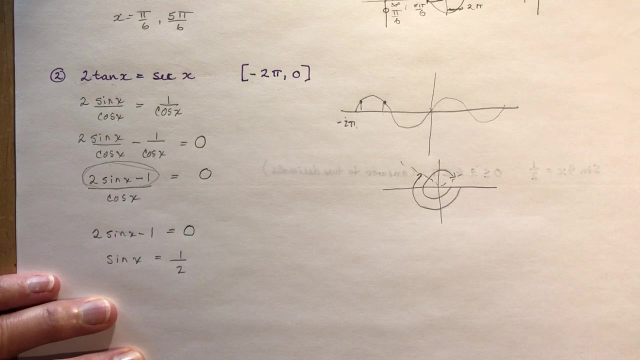 Negative angles. Negative angles go this way. so where is sine x? equal to half would mean I'd have to stop here and I would have another one over here. So there's one and there's two. Okay, so that's what. now you need to find the value that's going to mute my computer. 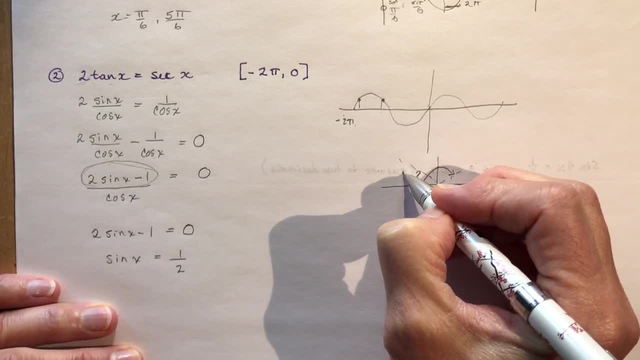 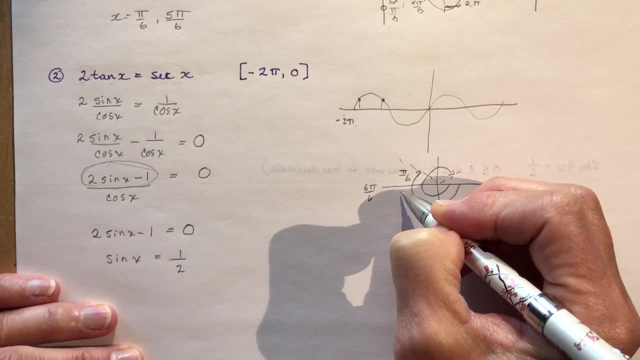 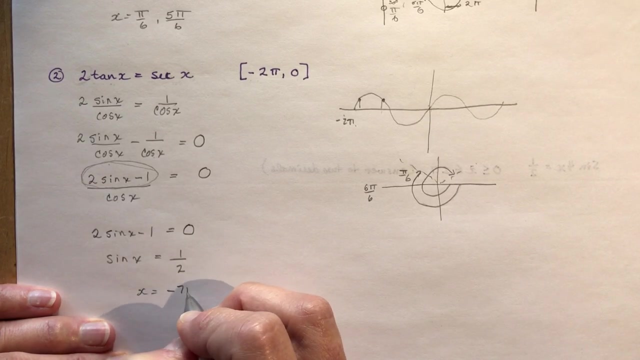 Okay, so this angle from here to here. Remember this is going to be pi over 6 and this is 6 pi over 6.. So this is going to be minus 7 pi over 6.. Remember going negative. So x is equal to minus 7 pi over 6, and the other solution would be the one way over here. 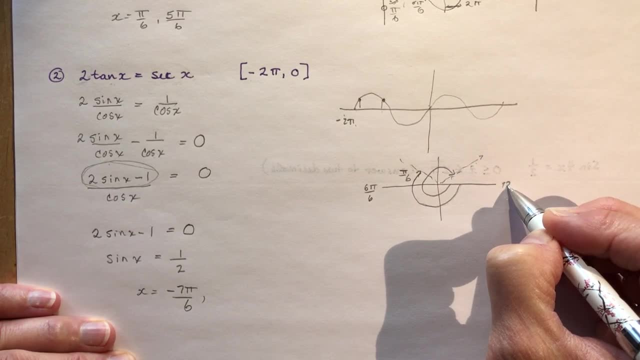 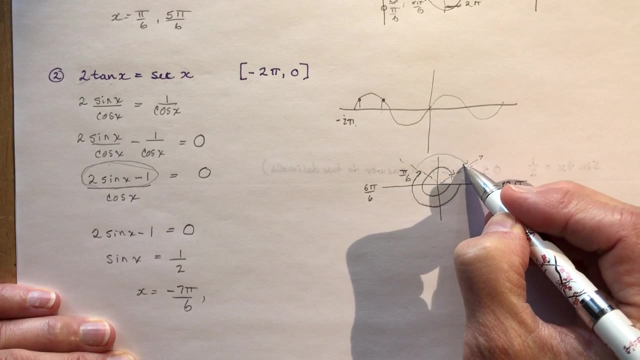 Now the easiest way again to do that is to say: oh, this is, this is 12, pi over 6.. So I'm going negative. So I'm going negative all the way Around to here. So that's pi over 6 is the related acute angle. 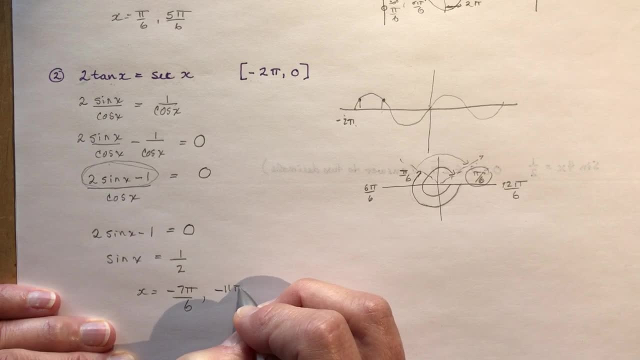 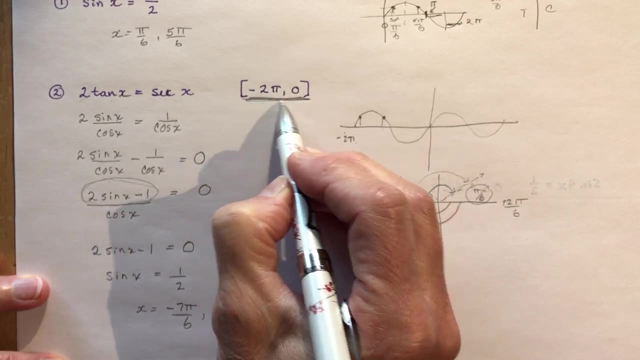 So this was going to be minus 11 pi over 6.. So you want to make sure, when you're done, that you're matching the domain restriction that you were given. So you're looking for those solutions and it's always nice to draw a little picture. 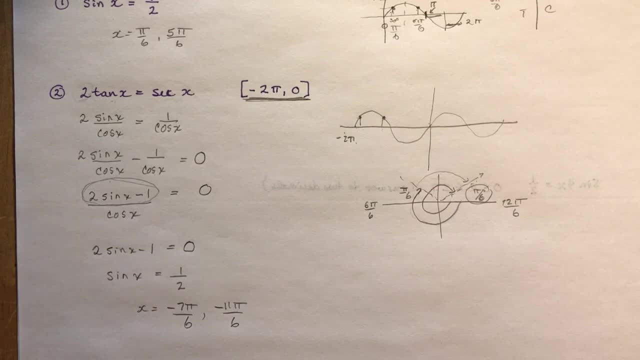 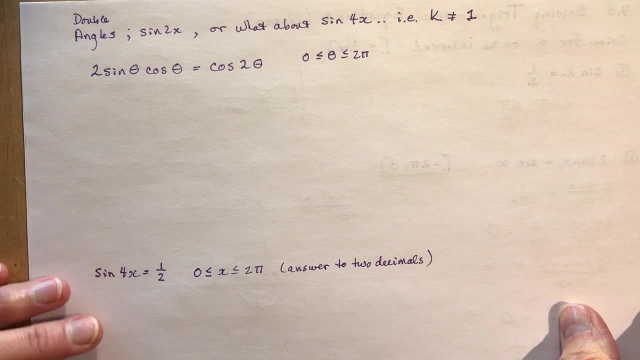 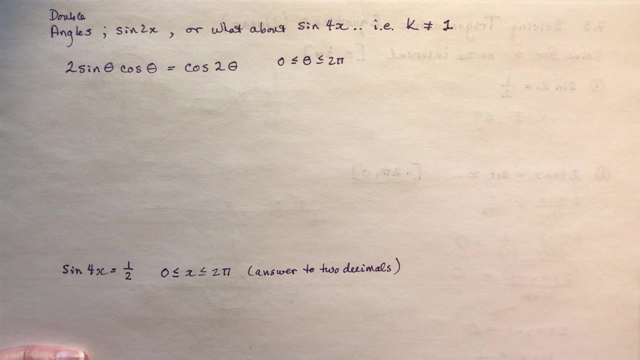 It helps you see where you should be. Okay, let's move on to something just a little more difficult, And that's when we have something Where k is not equal to 1.. So, in other words, when k is not equal to 1, we're changing the the period of the function. 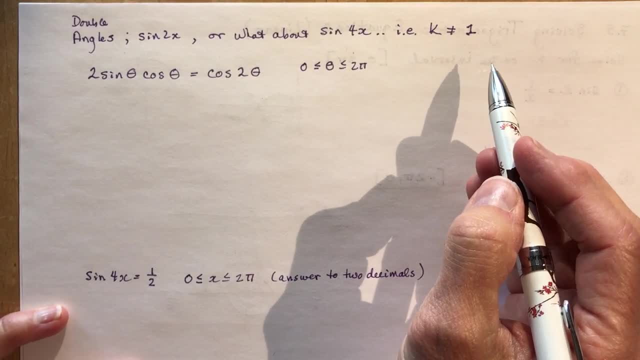 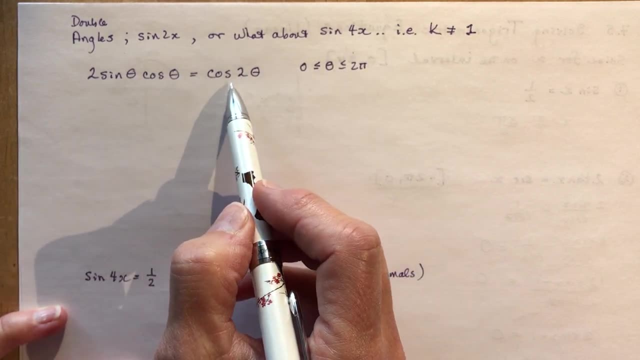 right, You know, you know that. you know that by now you know these lessons well. So this one who 2 sine theta, cos theta equals cos 2 theta. So again, like I said, you want to get a number on this side. 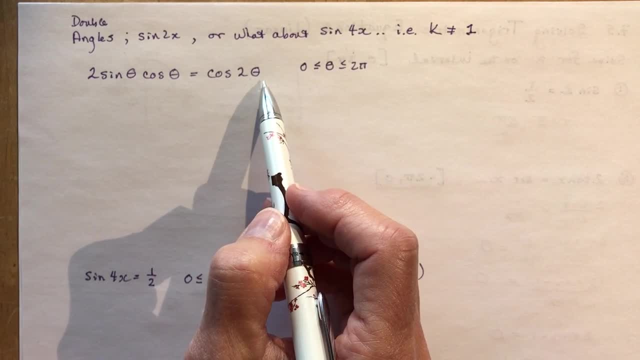 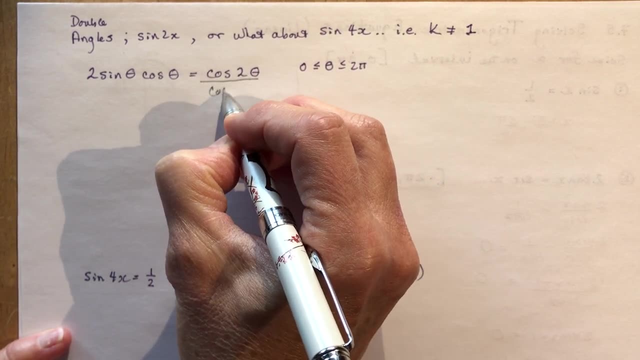 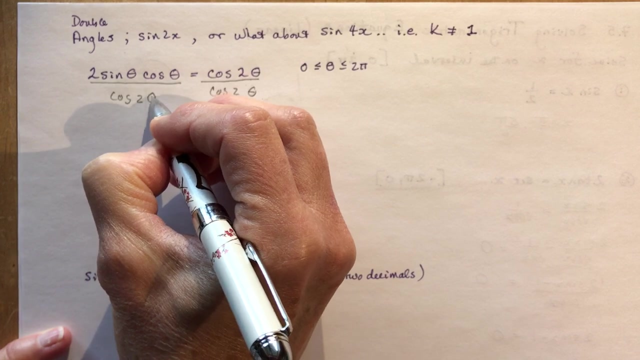 Now you may. you may make the mistake of saying: well, if I divide by cos 2 theta, which you can do, let's do that first. Let's say cos 2 theta And cos 2 theta Now. 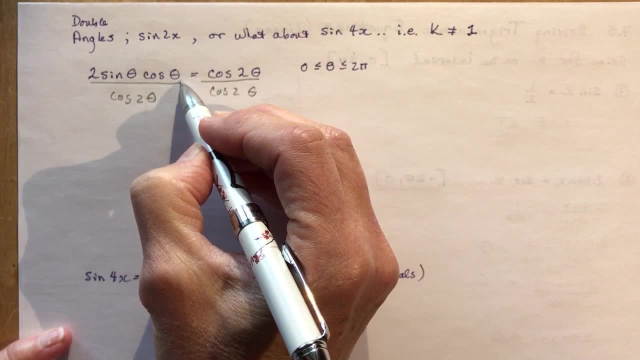 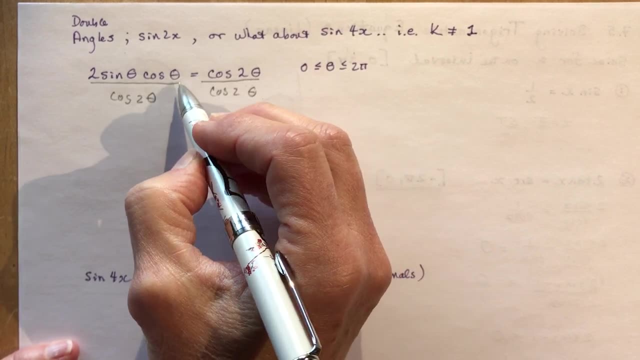 if you had subtracted this on the other side, then you would have been in real hot water, because you have nothing left to do with it. So sometimes you'll find you hit a roadblock. So go back, because if I had said this, 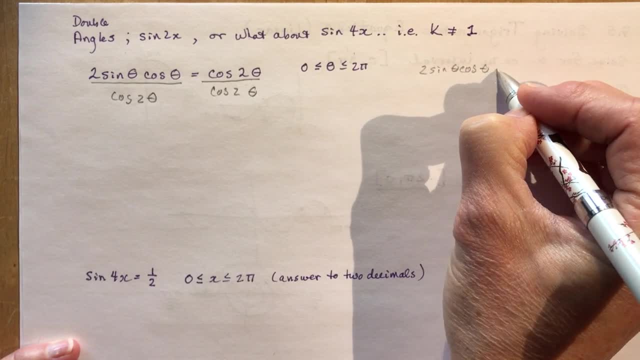 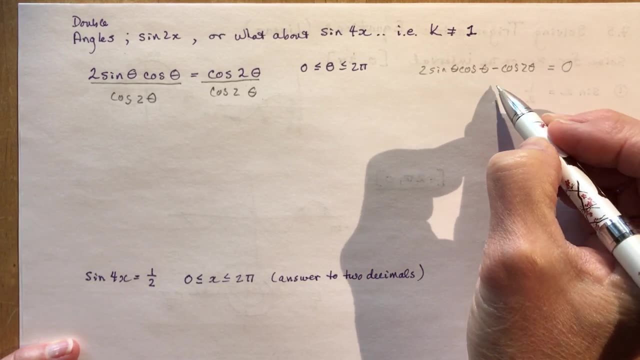 let's say I did this first. I said, okay, well, the last time we just subtracted it And I did this. And you'd say, oh, how am I going to? I can't factor cos theta out of this. 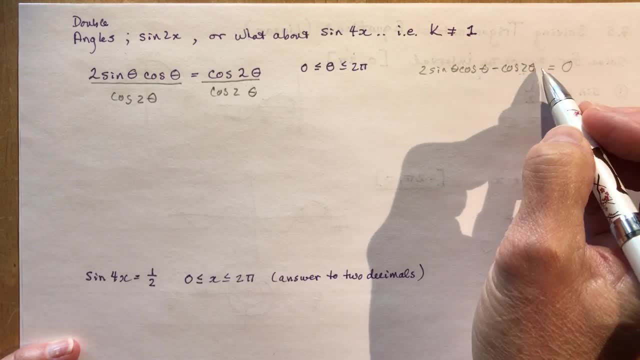 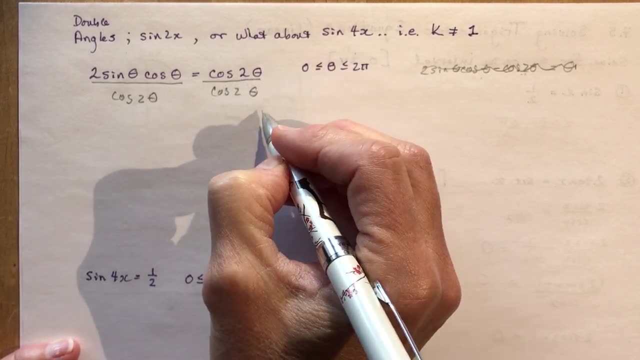 And then you might try to switch this to another format and it's just going to go messy. Okay, so divide by cos 2 theta, That's going to give me a 1 here. That's nice. What is 2 sine theta? cos theta though? 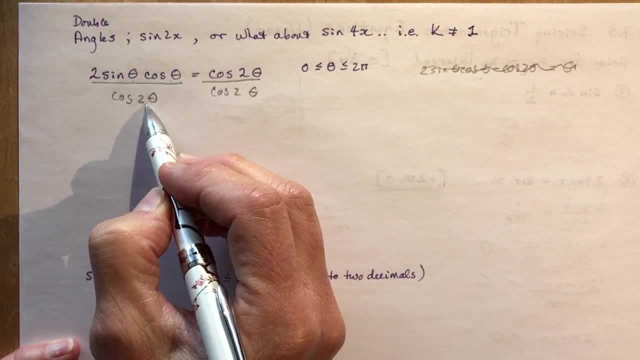 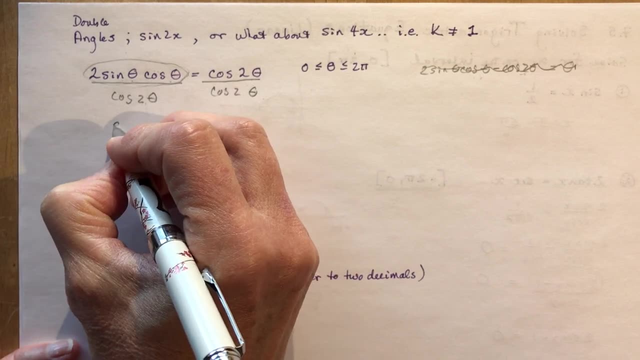 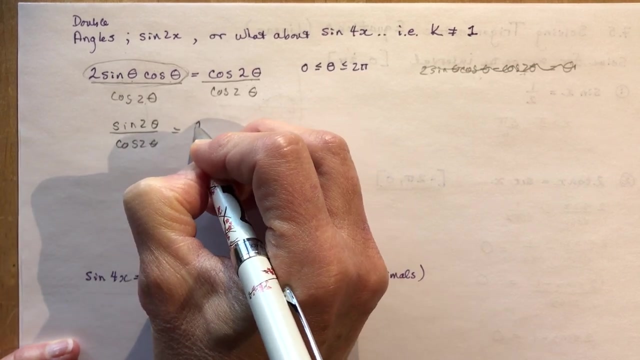 Well, because I can't really simplify this unless I do something up here And you should be saying: oh, 2 sine theta, cos theta, that's sine 2 theta, magic right, Sine 2 theta over cos 2 theta is equal to 1.. 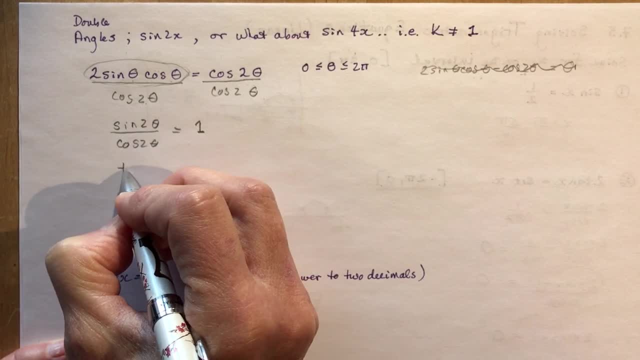 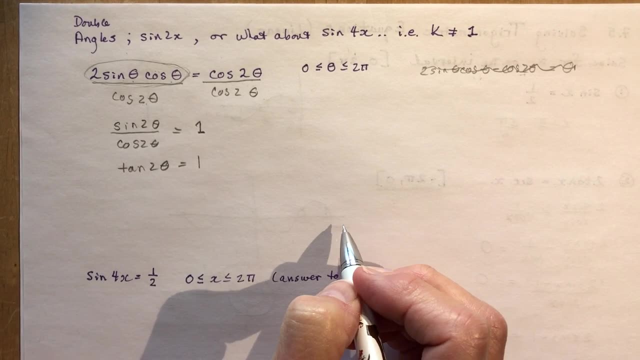 Now we're getting somewhere. So sine over cos that would be tan of 2, theta is equal to 1.. Now this is where you have to be careful, because if I use my calculator, you shouldn't need a calculator, because you know. 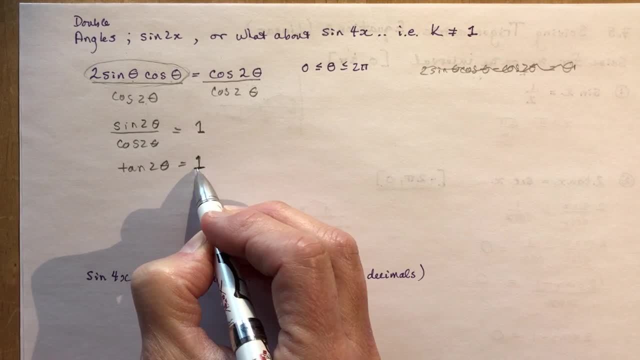 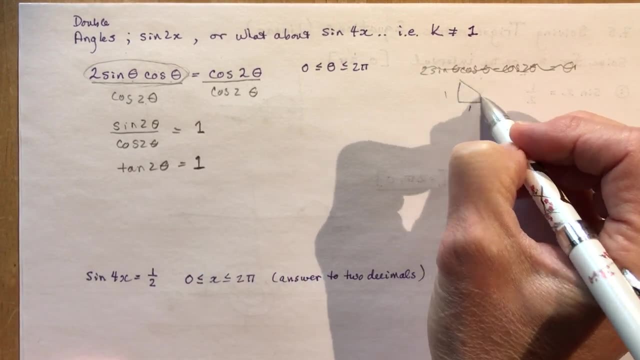 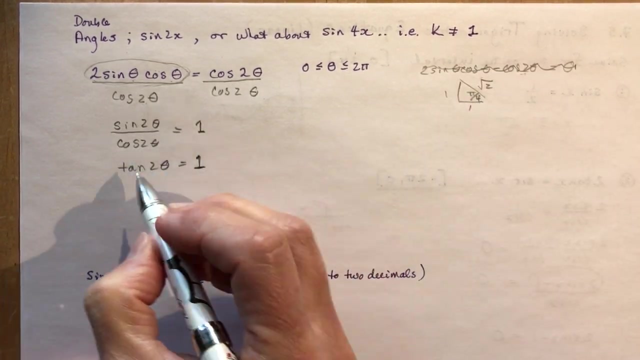 tan of theta is equal to 1 when theta is pi over 4, right 45 degree angle, That's your special one: 1, 1 square root 2. should be really good at finding that now, But if I do the inverse of this, 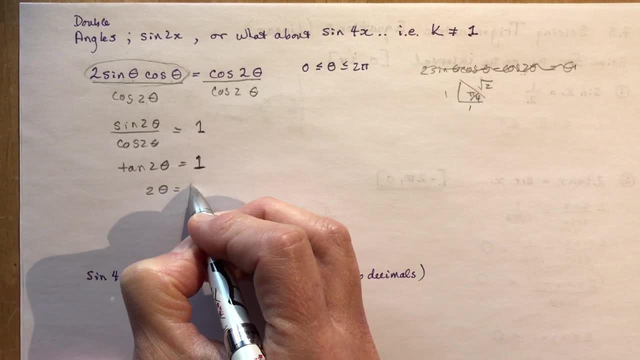 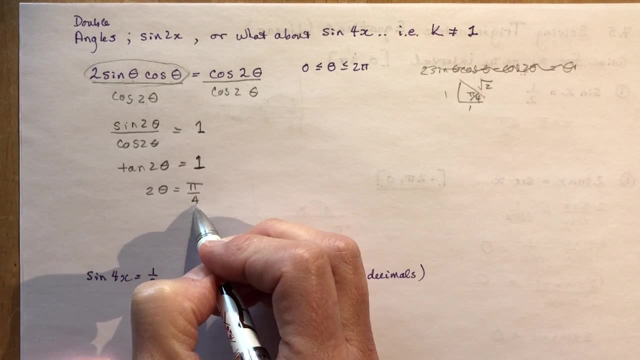 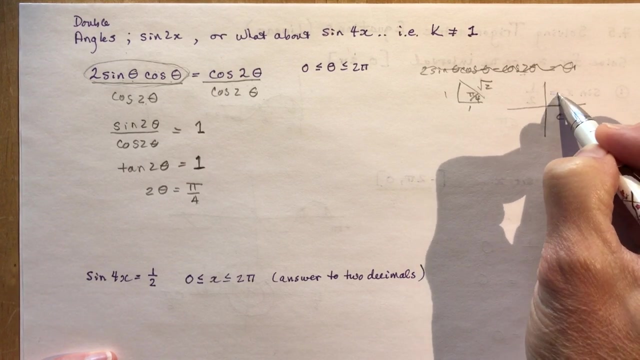 that would say that 2 thetas are equal to pi over 4.. Okay, now you're okay so far. you want to leave this one here and find the other place where theta is equal to 1. And that is in quadrant T here. 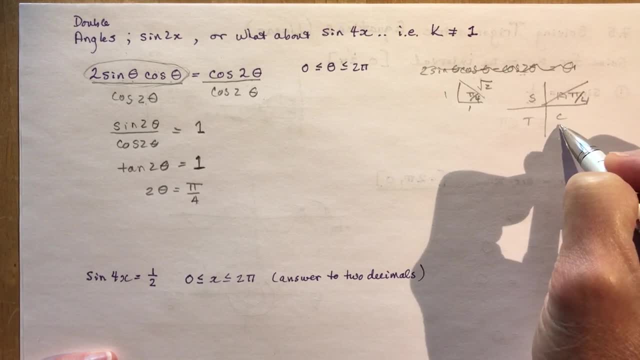 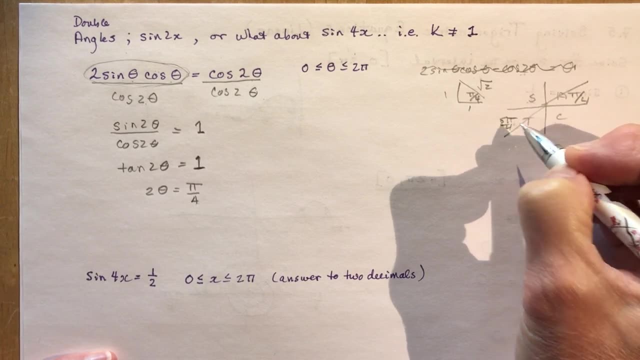 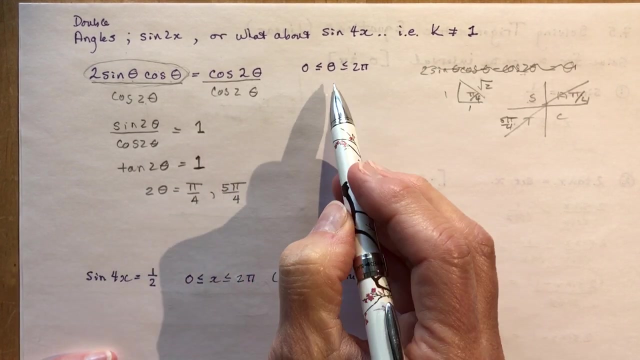 So I had pi over 4.. That's positive, positive one here and it would also be here. So this is going to be 5 pi over 4.. Okay, but the question asked me you're asked to find for theta. 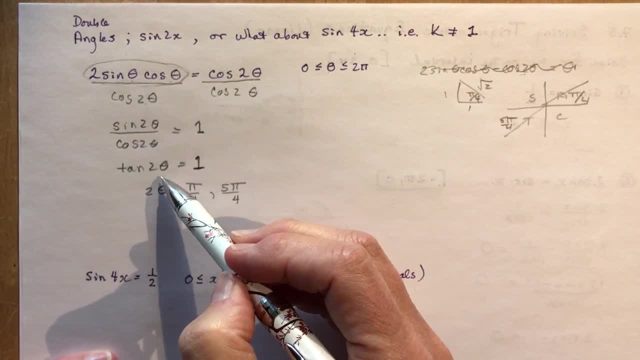 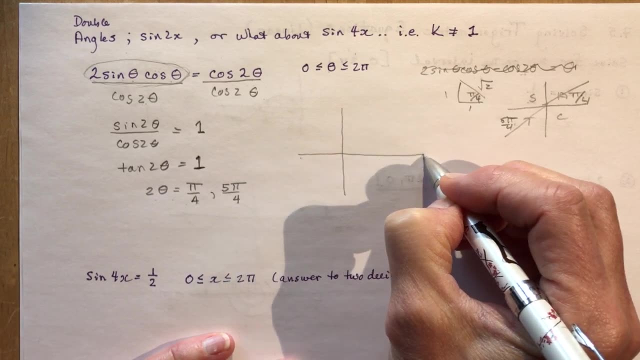 not 2 thetas. So you know that when you have tan theta, do you remember what the tan graph looks like? We'll sketch it It's. it's this wiggly one, Remember, and it had pi over 2,. 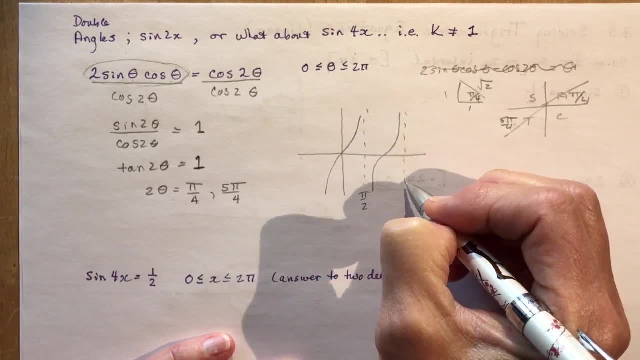 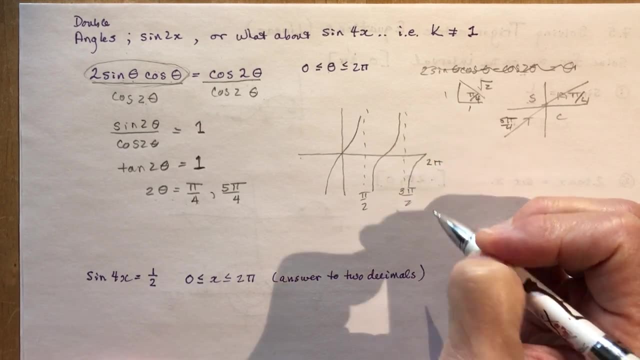 and then it goes through here again and then it has another asymptote at 3 pi over 2, and then it goes to here to 2 pi. So I want to know where tan 2 pi equals 1, and we found these two places here. 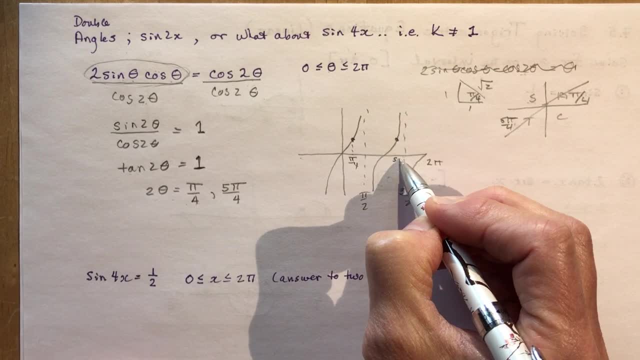 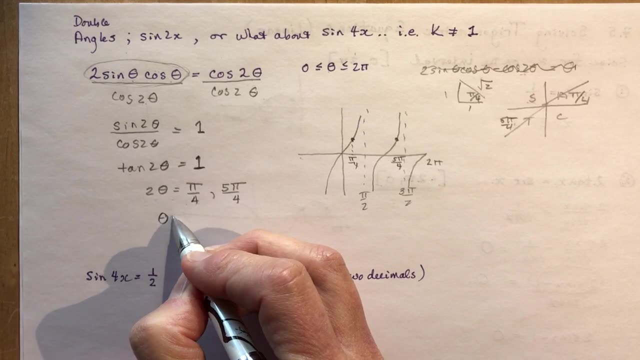 which is pi over 4, and this one over here which is 5 pi over 4.. But that's not the question. It says 2 theta. So what's theta equal to? Well, I just have to divide by 2,. 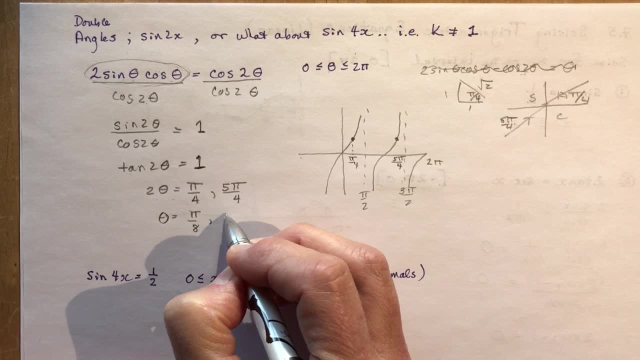 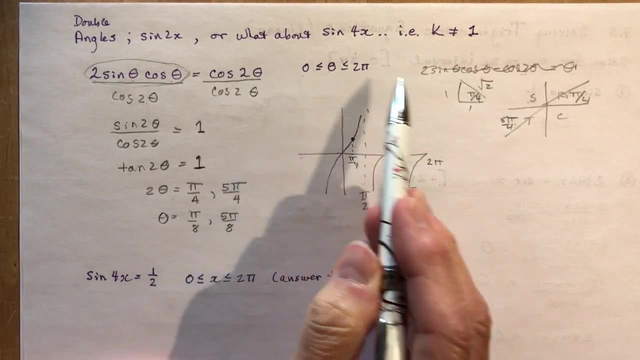 and that's going to give me pi over 8, and 5 pi over 8.. Now the problem is that I need to know between 0 and 2 pi. So this would be tan theta. right, This is tan theta. 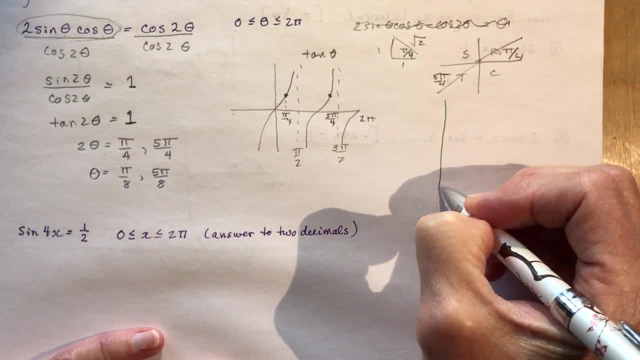 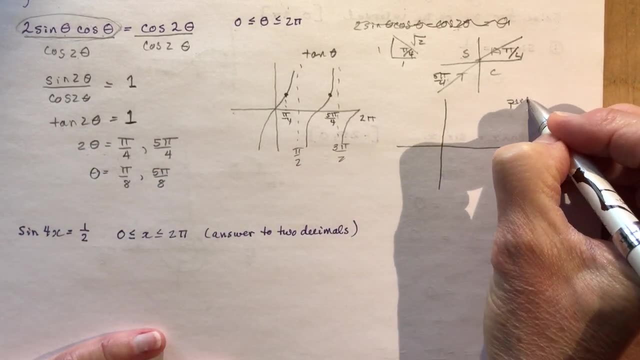 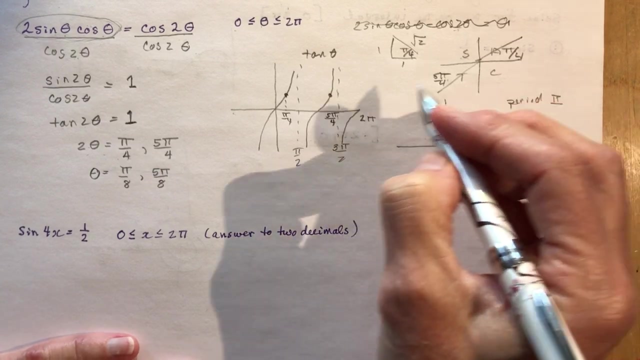 not tan 2 theta. So if I do tan 2 theta, what's the period? The k is 2.. So the period period is going to be pi over. remember the period of a regular tan function is pi right. 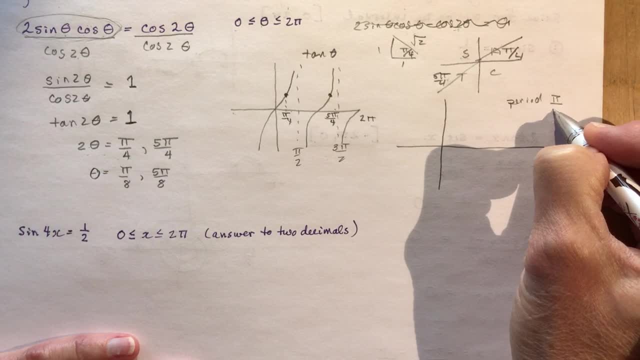 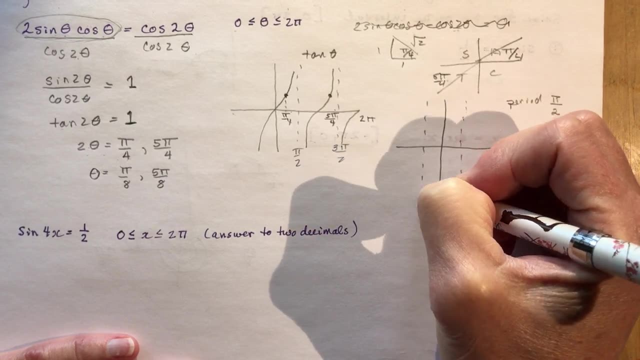 from here to here It's 180 degrees or pi, So pi over 2.. So that means that this asymptote here is going to be half of where this one was right. So this is going to be pi over 4,. 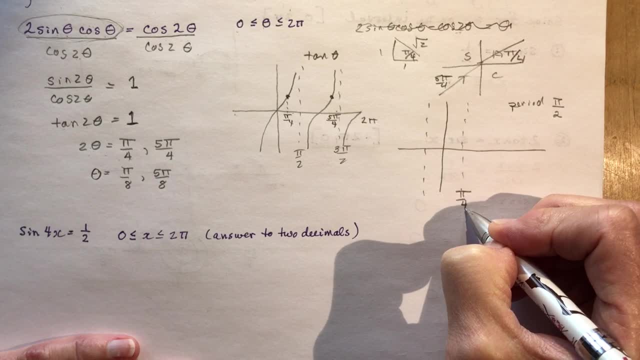 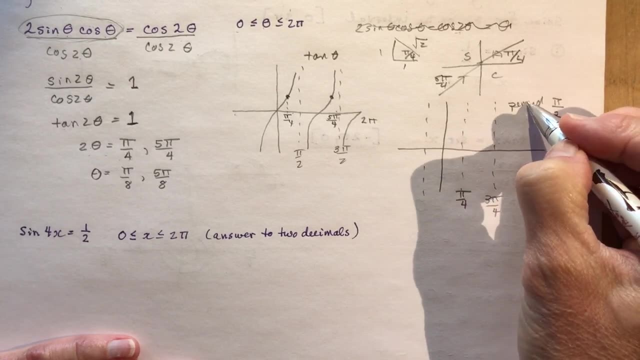 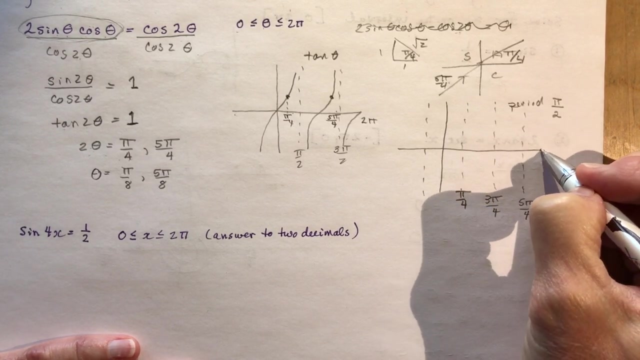 and the next period is going to be at 3 pi over 4.. Next asymptote: sorry, this is going to be 3 pi over 4.. Add two more: you're going to get 5 pi over 4, and 7 pi over 4.. 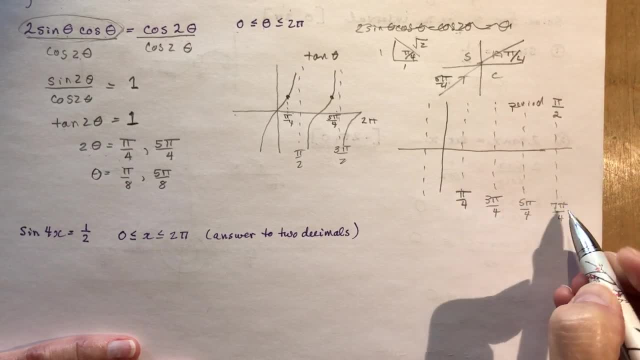 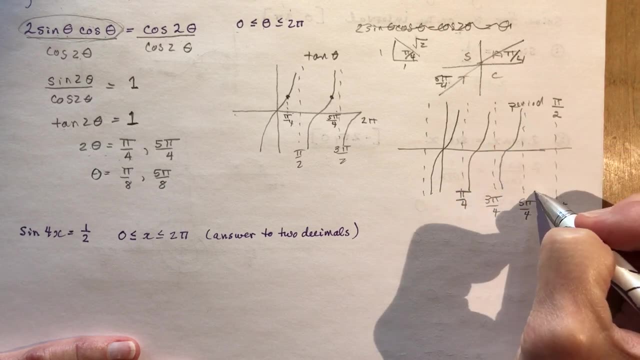 So just keep adding 2 pi over 4.. So here we go. Now we've got our tan. function is going to go like this now, And you're going to see that there's 8 pi over 4, or 2 pi. 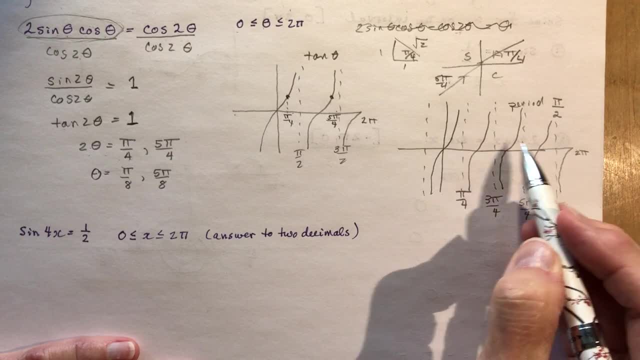 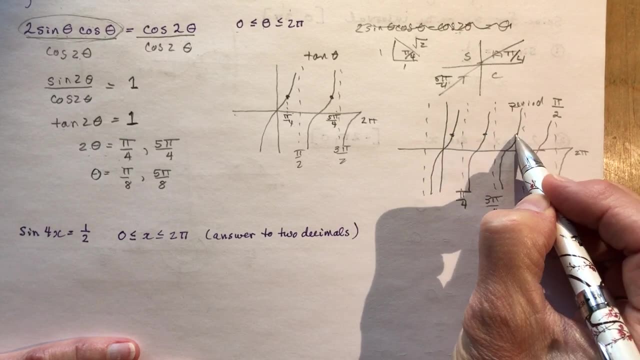 You're going to see that you actually have, because this is a horizontal compression right. So we have. we have more values where it's going to be equal to 1.. So we should have 1,, 2,, 3,. 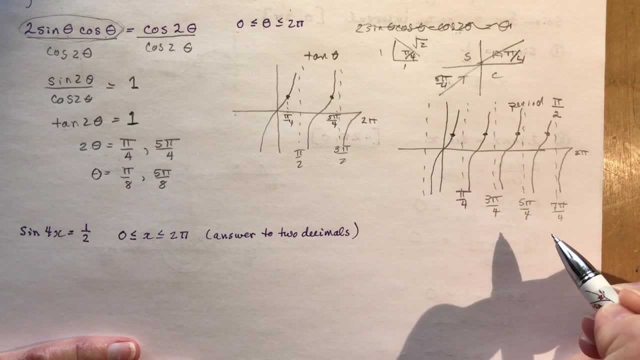 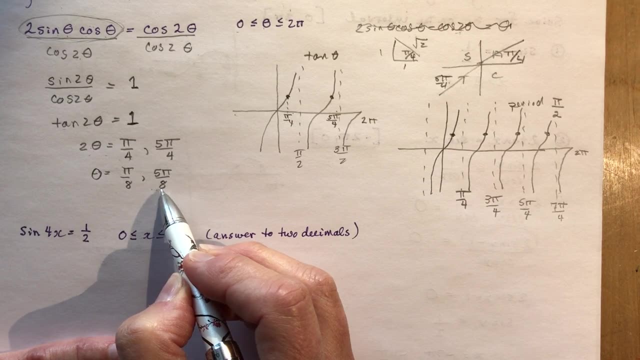 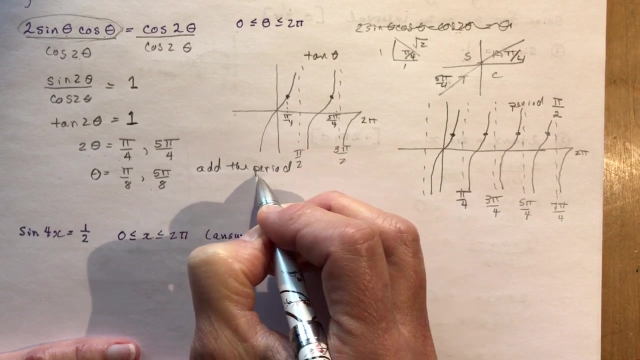 4 solutions. So if I found these two solutions, all you have to do now is add. we're going to add the period. Add the period until I get close to 2 pi. Don't go over it, right, Because that's my domain here. 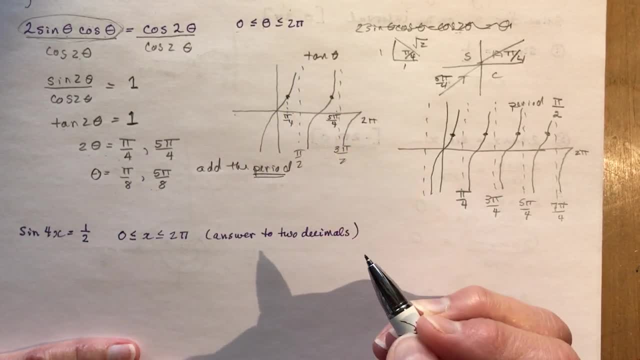 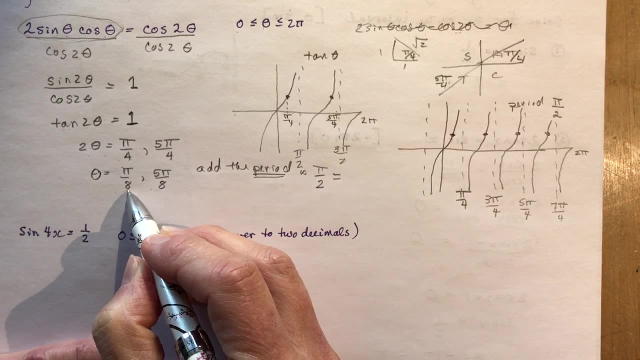 0 to 2 pi, And what is the period? The period is pi over 2.. The period is pi over 2, or I'm going to write it with a base of 8, because I'm adding it to these fractions anyway. 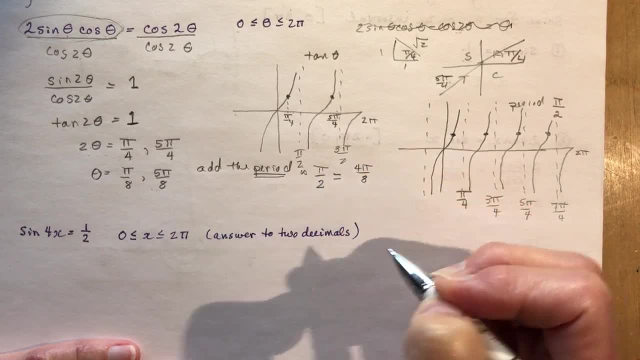 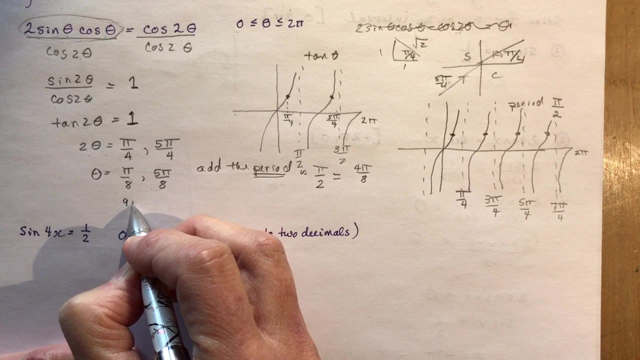 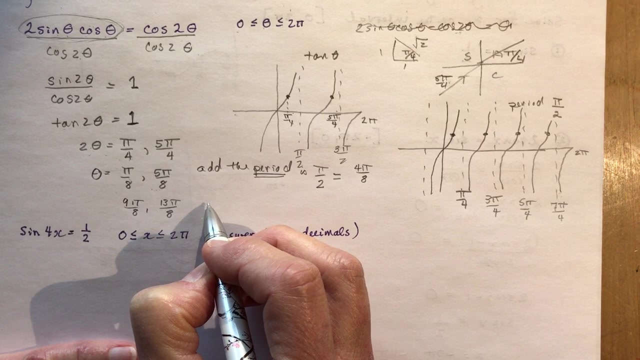 So that would be 4 pi over 8.. So I have pi over 8,, 5 pi over 8, keep adding 9 pi over 8,, 13 pi over 8,, 17 pi over 8? No, that's passed. 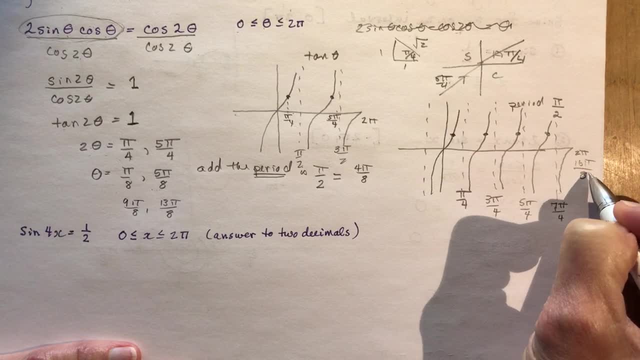 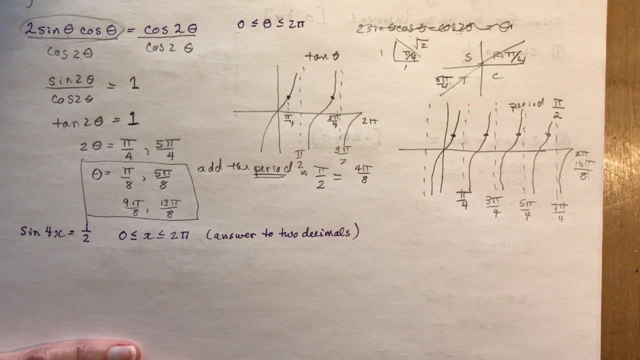 16 pi over 8?? That's this one here. right, That's 2 pi, so I have to stop. So here's my 4 solutions here. Okay, you might want to run over that one again, just to make sure that you've got it clear. 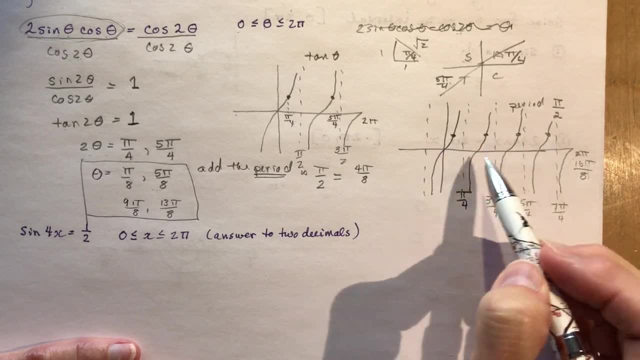 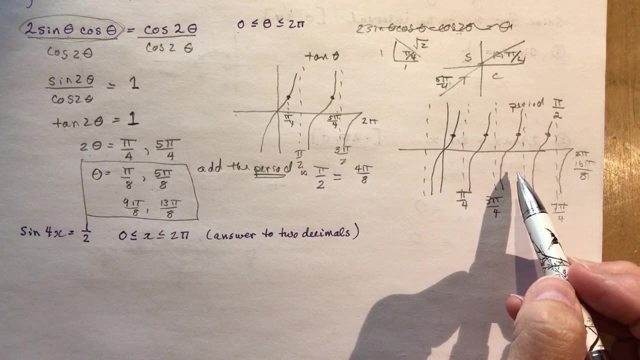 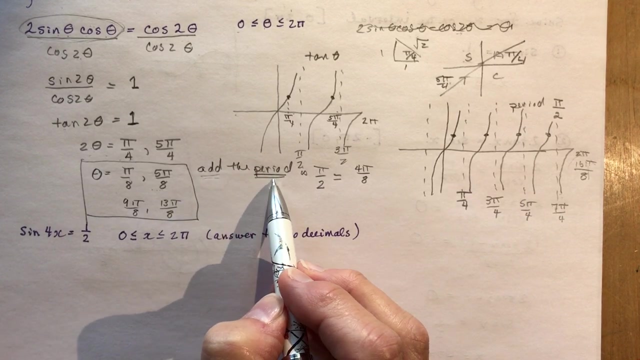 But it's helpful if you can make a sketch of the function, because that way you can see how many solutions you should have. If you can't sketch the tangent function, just knowing that you keep adding the period, add the period. that's very important. 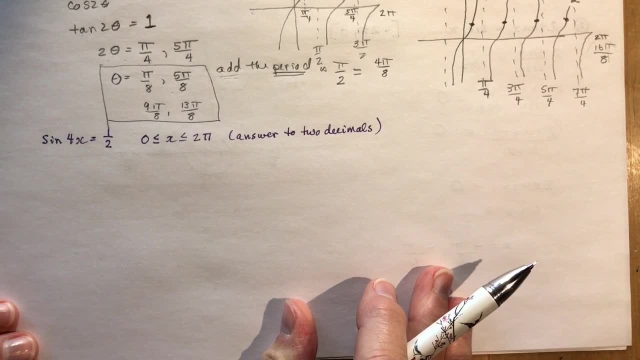 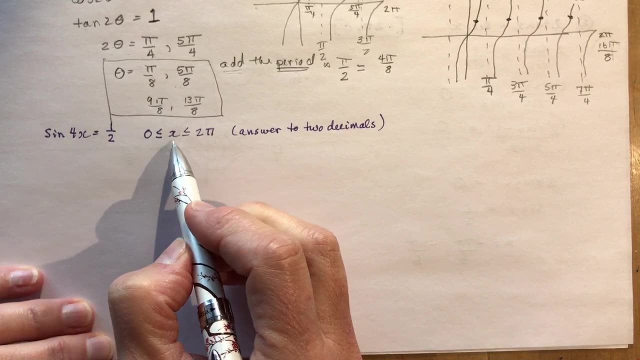 We're going to do that again with this question here, and hopefully by the time you've done this one you'll have it all figured out. Okay, nice one. Sine 4x equals 2: 1⁄2, where x is between 0 and 2 pi. 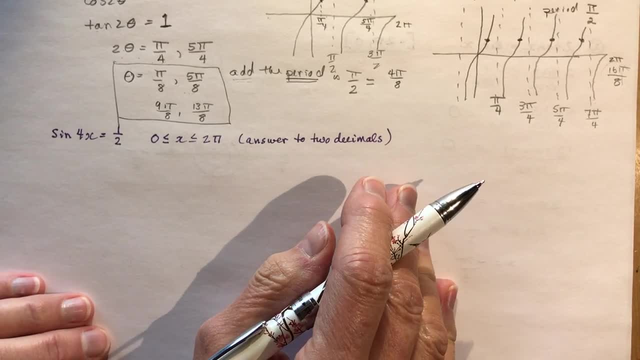 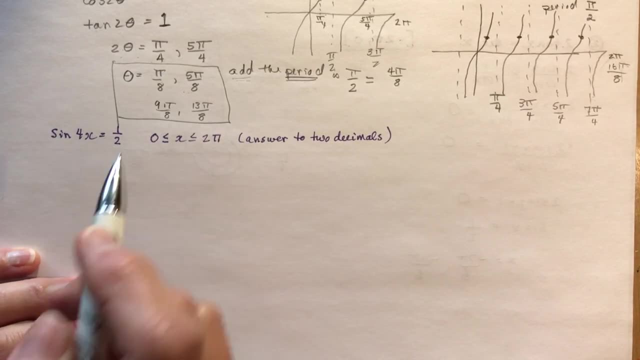 answer to two decimals. Okay, this is read out of your textbook. So, instead of giving me the answer of pi over 6, for sine x equal to 1⁄2, I need to use my calculator. So let's go here. 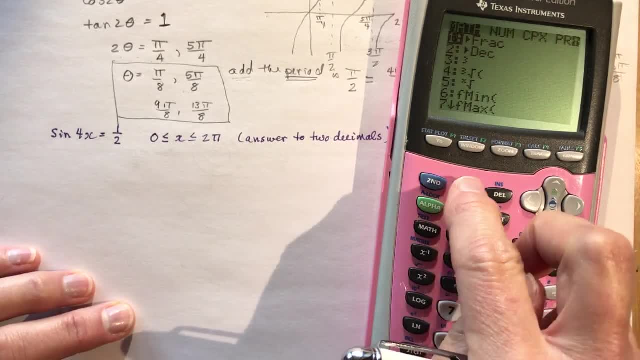 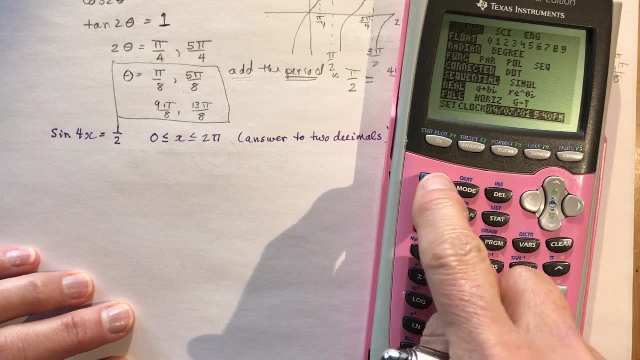 So make sure you're in the right mode here. right Mode radians, Okay. always double check that. It's a big problem if you don't, Okay. so I want to know. I want to know: where is sine x equal to 1⁄2.? 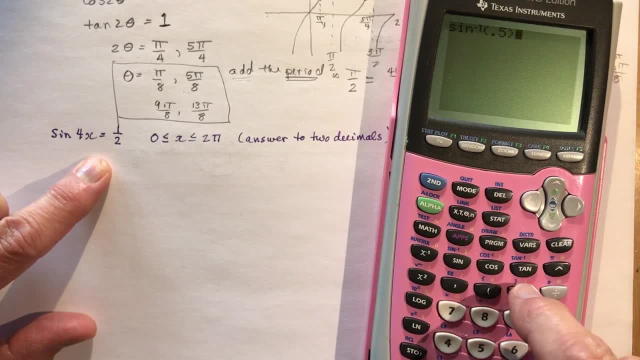 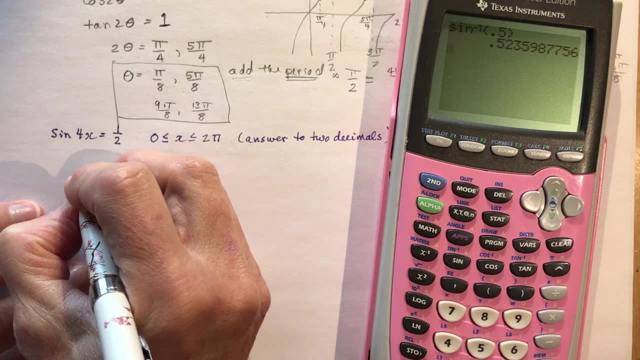 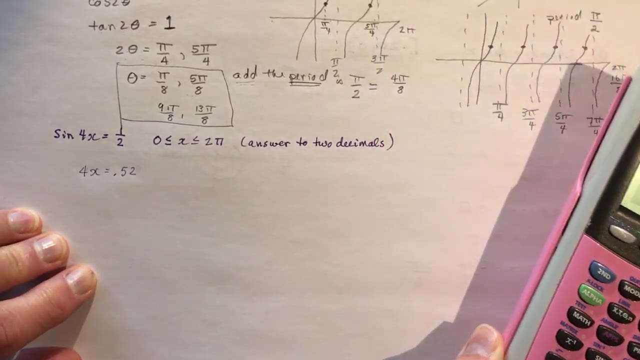 So second sine of 0.5 equals, and I get 0.52.. It says to two decimals, so 0.52.. So 4x is equal to 0.52.. Where's the other solution though, Because you know you have two? 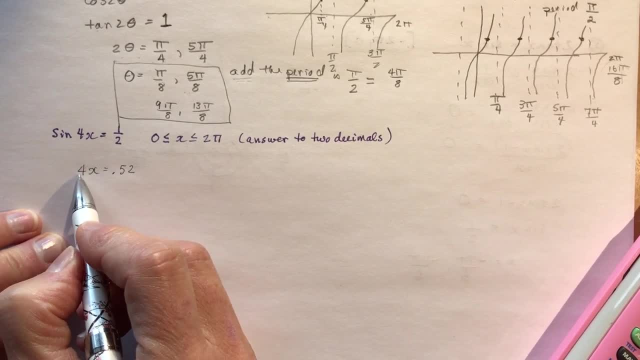 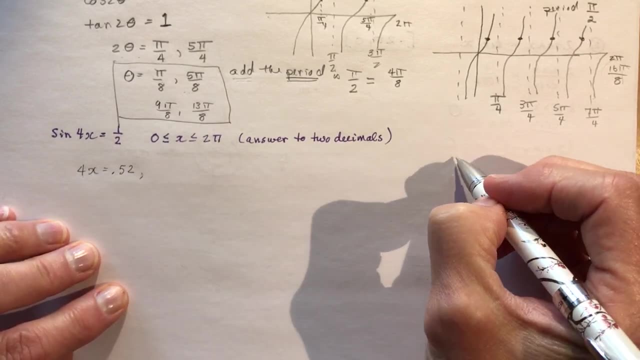 Between 0 and 2 pi. Just ignore this 4 for now. Okay, just ignore it. So 4x is 0.52.. The other place where you're going to have sine x: 1⁄2.. So we have here and here, right. 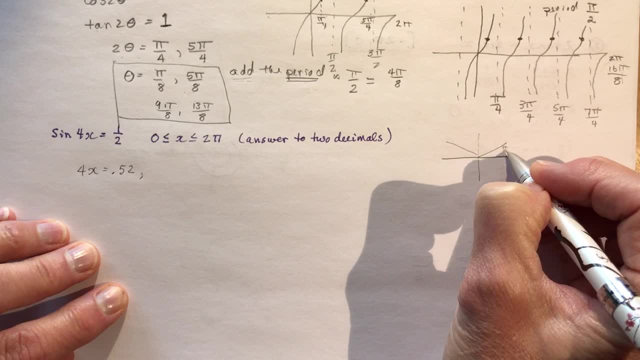 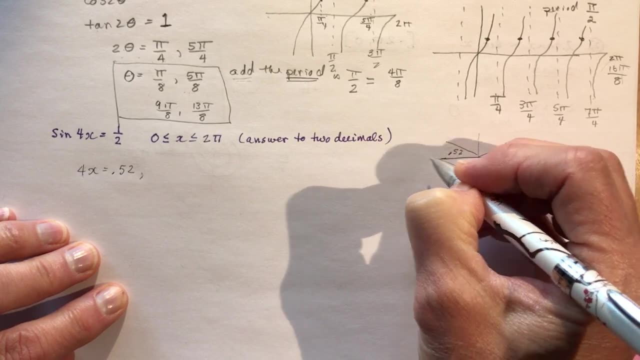 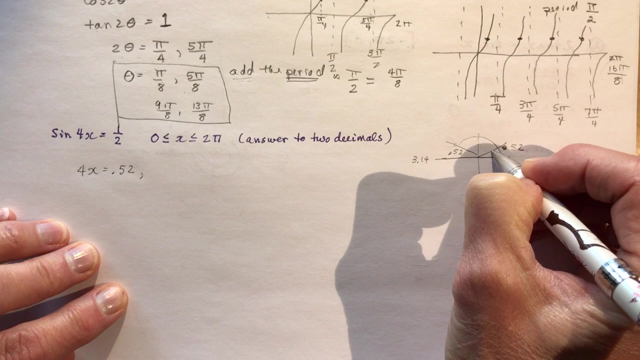 So this was pi over 6, or we'll use the decimal, So 0.52 radians, So this is 0.52.. And this is 3.14.. So I want this distance here, So this is one of my solutions. 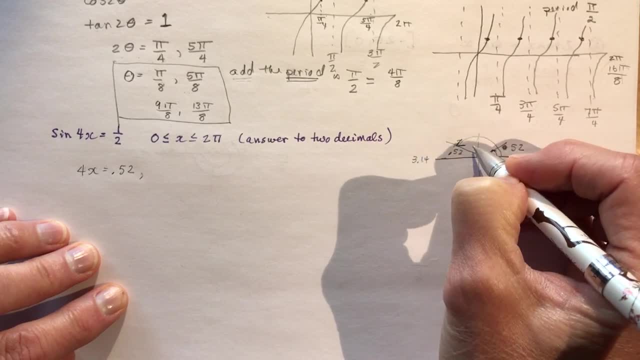 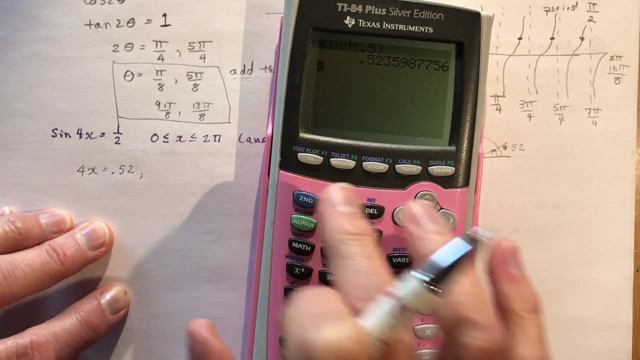 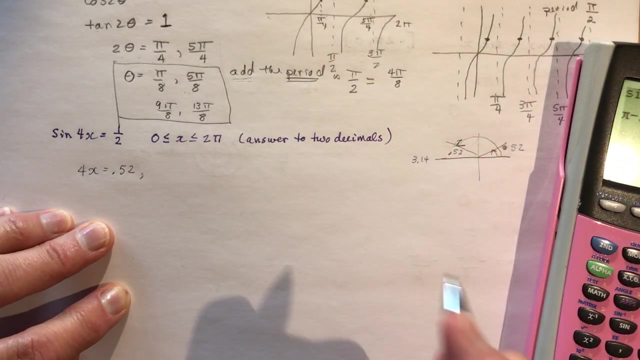 That's 0.52.. And the other one is this one all the way over to here. So I'm going to do pi minus 0.52.. So I do pi minus 0.52.. And I get 0.262.. 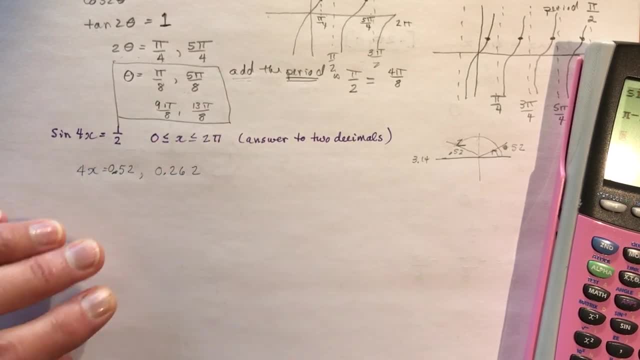 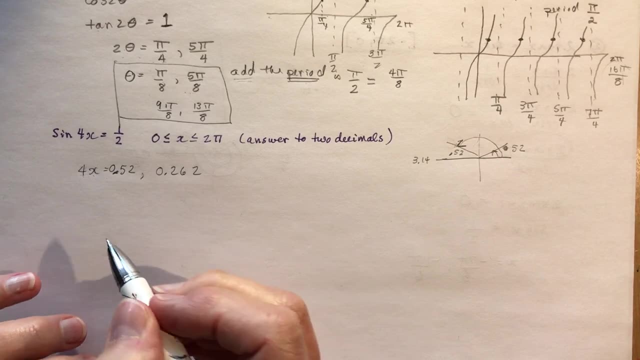 0.262.. You should put a 0 first, It's nicer. Okay, Now this is 0.2.. This is where you stop and you change this to 1x. Sorry, I got a bit of a cold today. 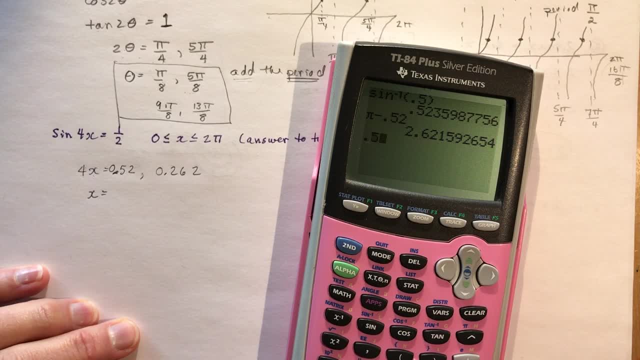 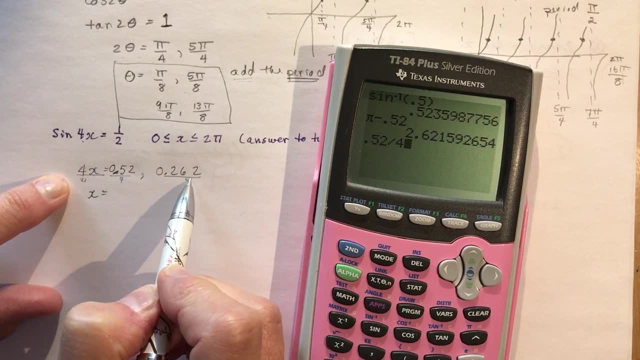 So x is equal to 0.52.. So I'm going to 0.52 divided by 4.. Because there's 4 x's Divide by 4, right 4 divided by 4 divided by 4.. And I get 0.13. 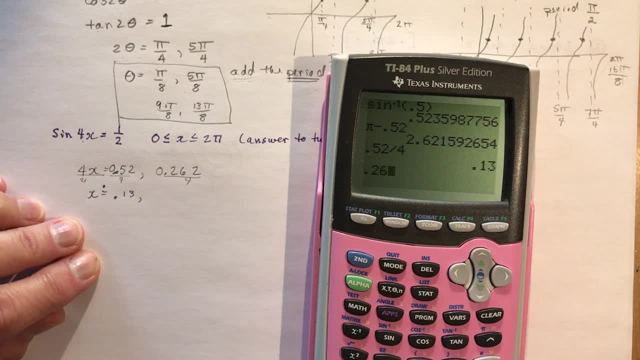 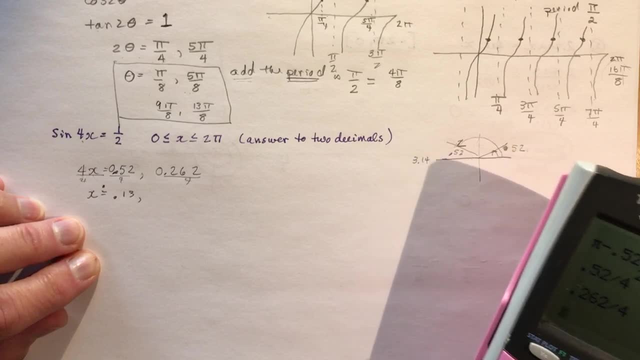 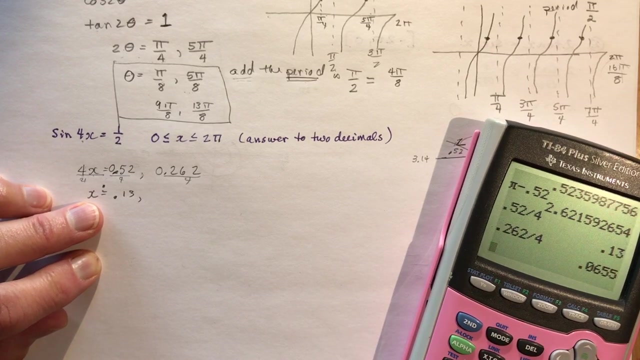 These are approximate values, So you might want to note that 0.262 divided by 4 gives me 0.. 0.262.. That's not 0.262.. 3.14 minus 5, 2.. I must have put a decimal in the wrong spot. 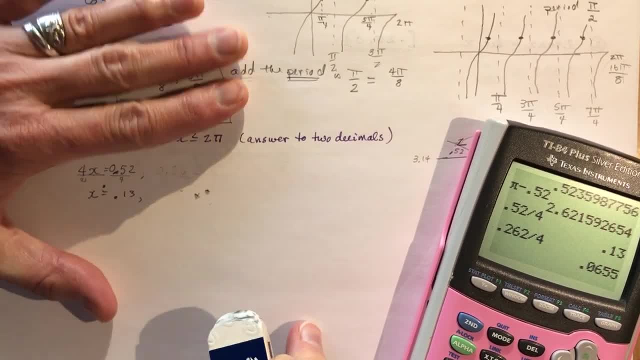 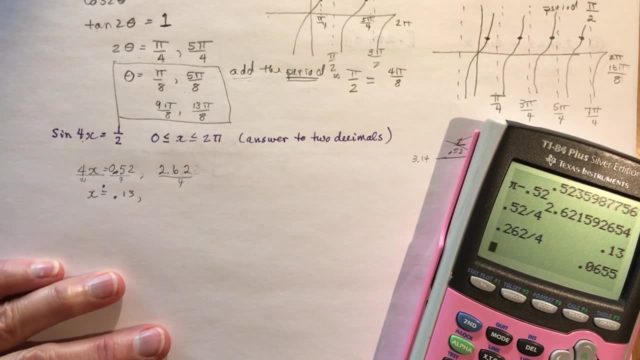 It doesn't make any sense at all: 2.62.. It even says that on your calculator, Ms Havrat. Okay, Divide that by 4. And that's going to give me. Well, let's just put it on here. 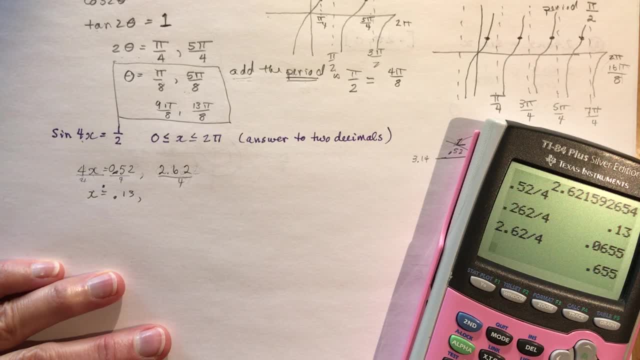 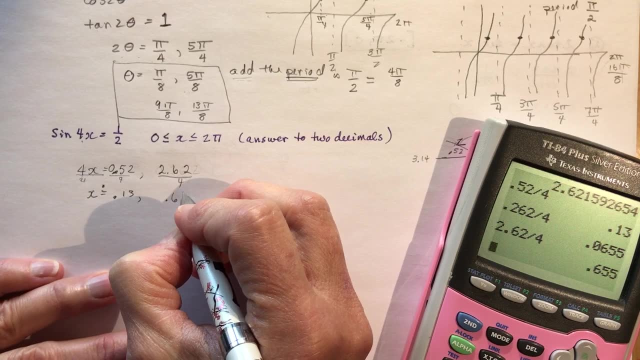 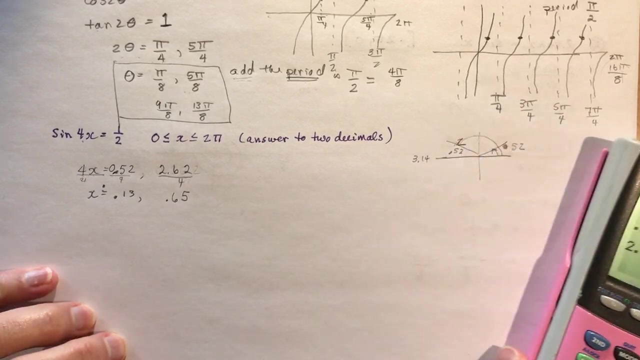 So 2.62 divided by 4. And I get 0.65.. 0.655.. We said only two decimals. Well, if I had left it as this long number, I would have got 0.65.. Okay, So there's two solutions. 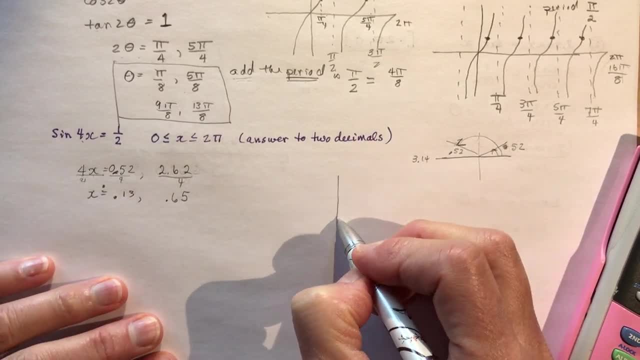 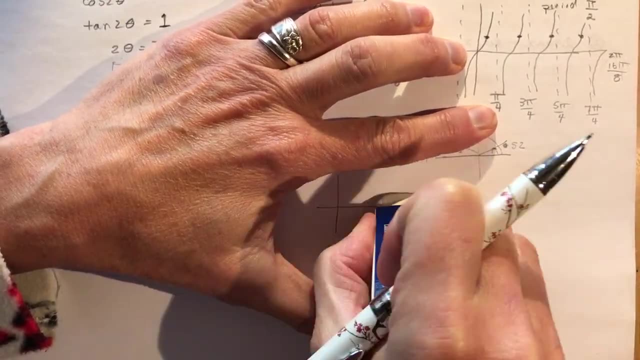 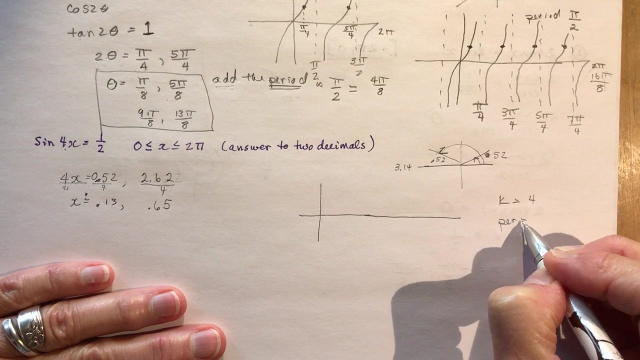 That's all you've got. Are there more? Absolutely, Because you know what sine 4x looks like. What's the period if k is 4?? k equals 4. Period equals 2pi over k, So the period is only pi over 2.. 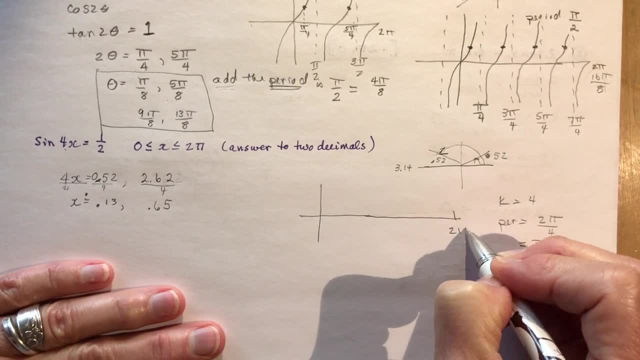 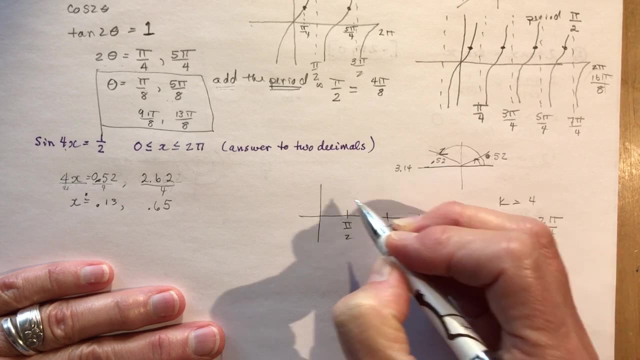 Oh my goodness, Pi over 2.. So in 2pi's Let's go pi. Here's pi over 2.. Here's 3pi over 2.. I have all these little sine functions. There's 1., There's 2.. 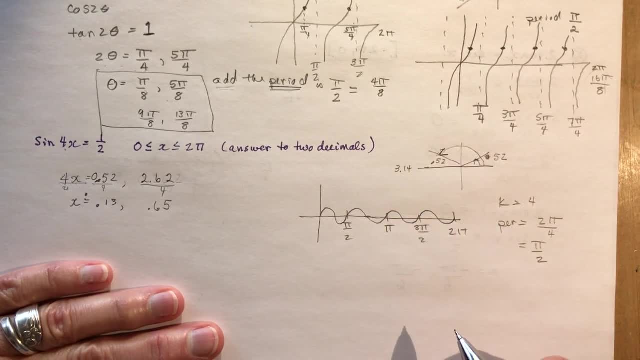 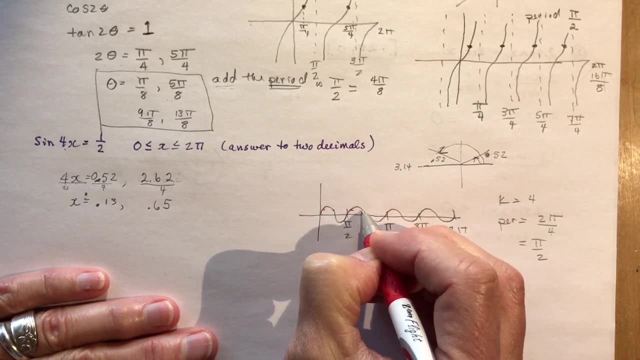 There's 3.. There's 4.. How many solutions am I going to have? So you want to look Where is it going to be equal to? It's going to be equal to a half. So 1,, 2,, 3,, 4,, 5,, 6,, 7, and 8.. 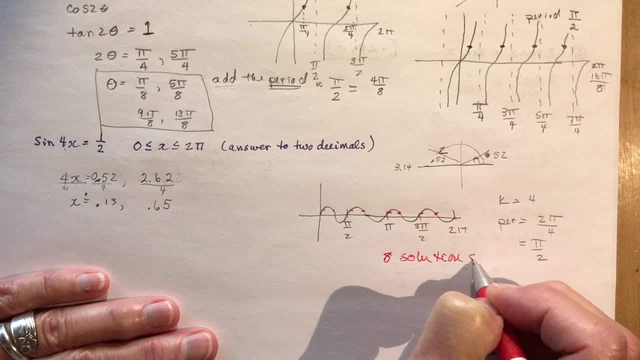 Eight solutions, Oh my goodness. Okay, How are you going to find those? Just like we did above, You want to add the period, So you want to add pi over 2 to each of these solutions until you get to 2pi. 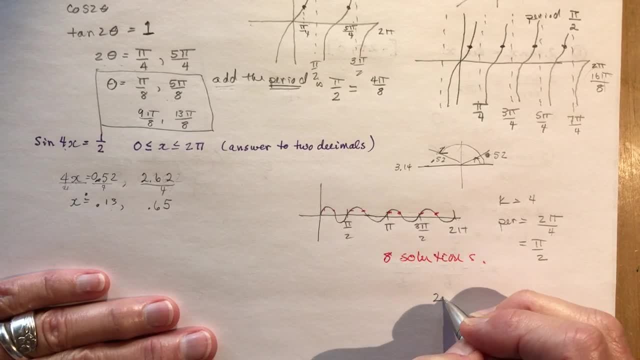 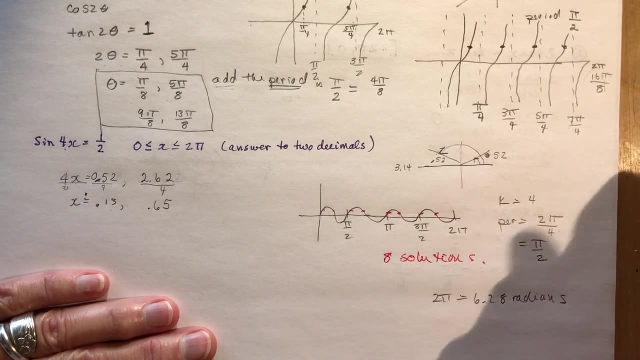 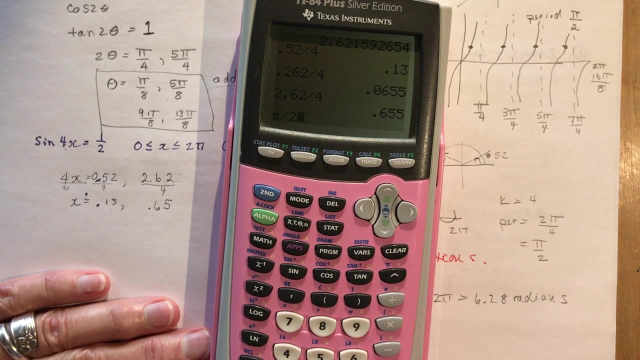 So 2pi is going to be 6.28. Right, 6.28. 8 radians, So if I'm adding pi over 2.. So let's go back here and find out what pi over 2 is Pi divided by 2.. 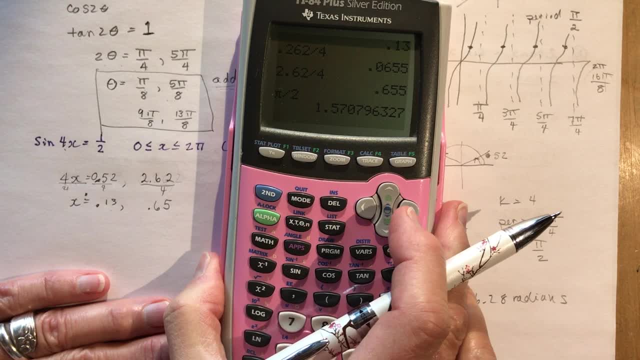 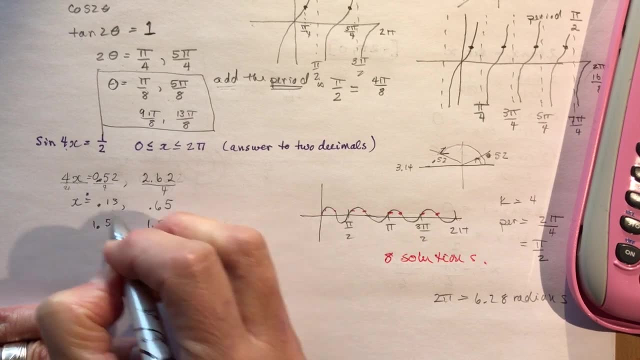 And I have 1.57.. So I'm going to add 1.57 to each of these numbers. So I'm going to just put a little box around our solutions. So we have this one and this one. Now we're going to add 1.57.. 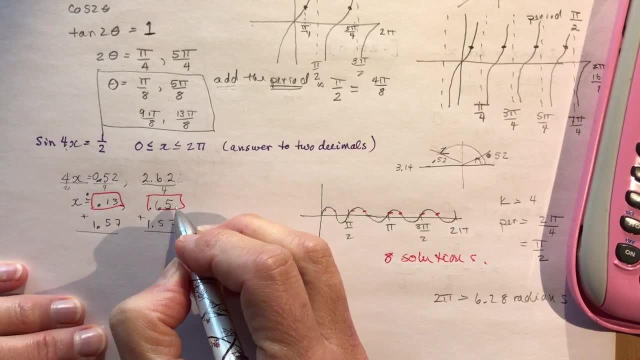 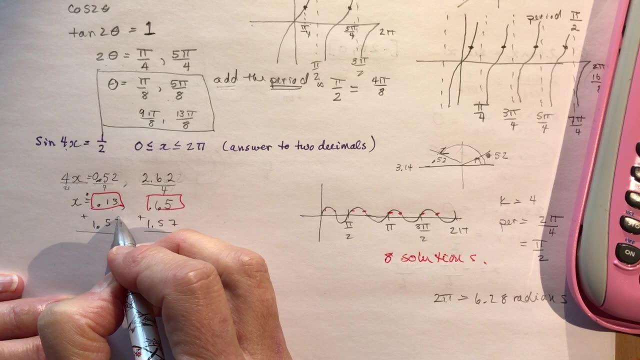 I'll put a plus sign here, so you remember: 5 and 7 is 12.. 6 and 6 is 12.. 1 and 1 is 2. 2.22.. That's such a nice number, 10.. 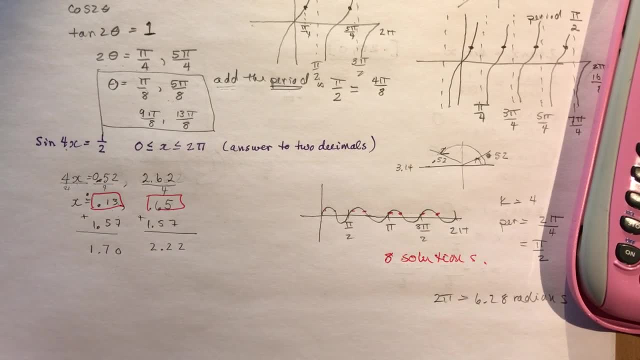 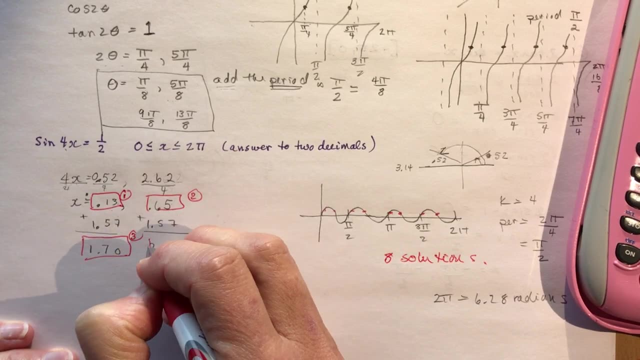 7. 1.70.. Okay, So this is my first solution. My second solution, This is my third, This is my fourth. So even if you can't sketch this, You would know that you have to get to 6.28.. 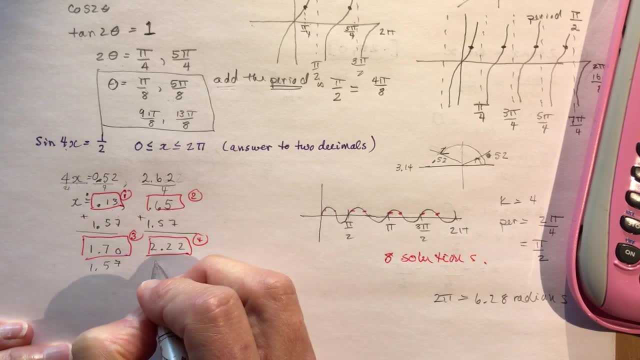 So you've got to keep adding 1.57.. 1.57.. That's 7.12.. 3., 9., 7., 3. And there's two more solutions, So that's 5.6.. 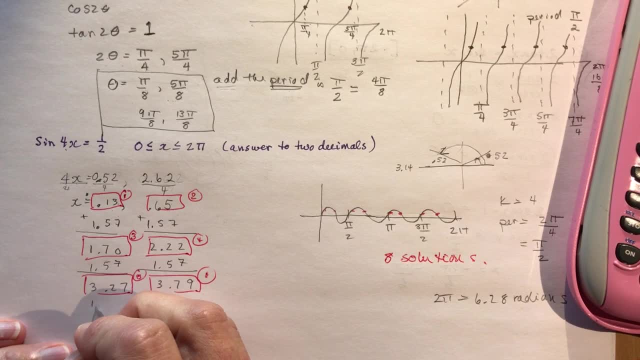 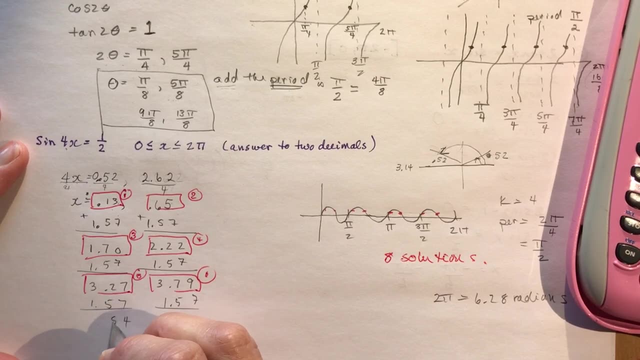 And add 1.57 again. Get good at adding. You shouldn't need your calculator for this kind of math, Right? 14. 8. 4. 4.8. 4. 6. 13. 5.36.. 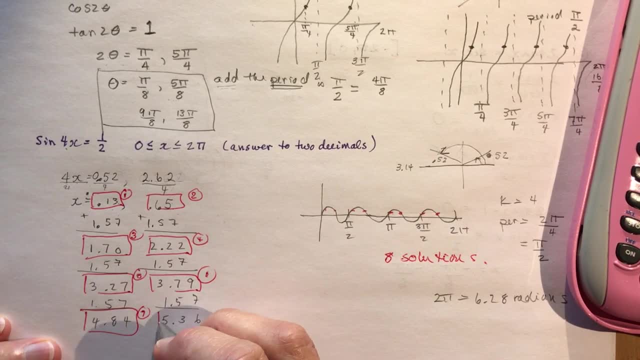 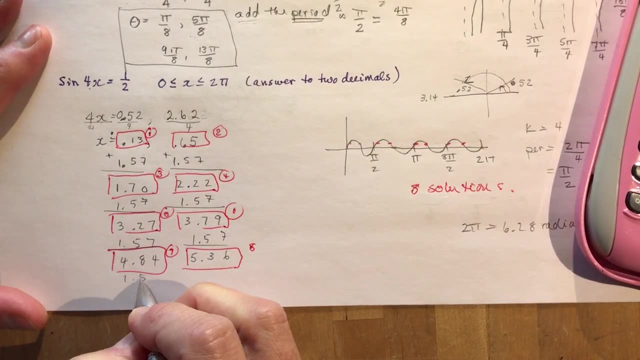 Okay, 6., 7. And this is my eighth solution. So if I added 1.57 to this, Let's just see what happens if we get 1.57.. 4 and 7 is 11.. 6 needs 14.. 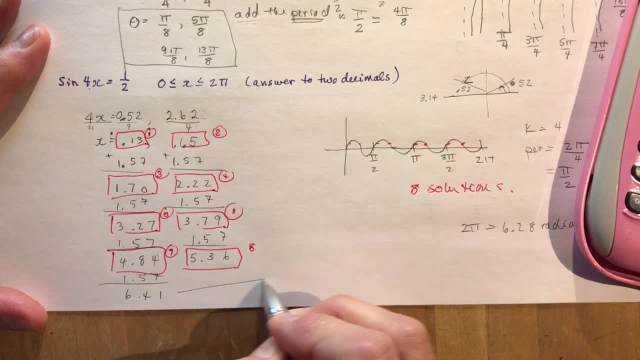 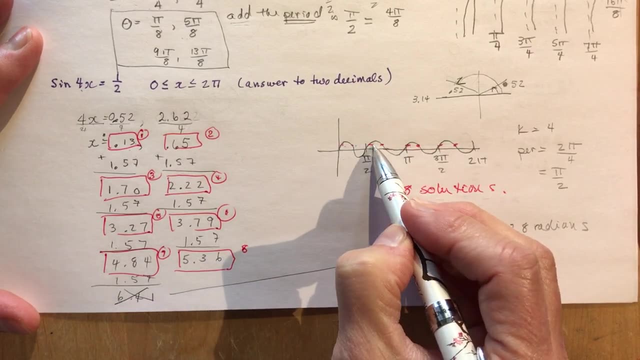 And 2 and 4 is 6.. Whoops, Look, We can only go to 6.28 radians. So this one is not a solution, And we've proven it by drawing this little graph for you. Okay, So I hope that helps you. 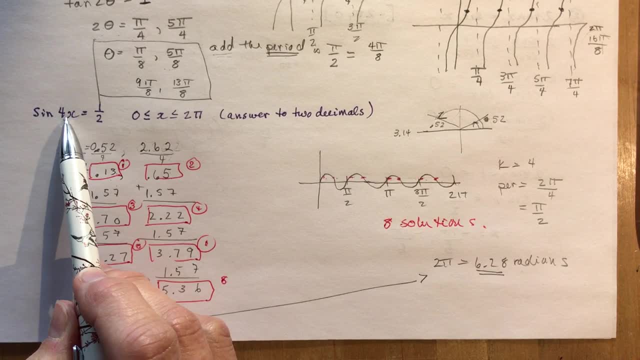 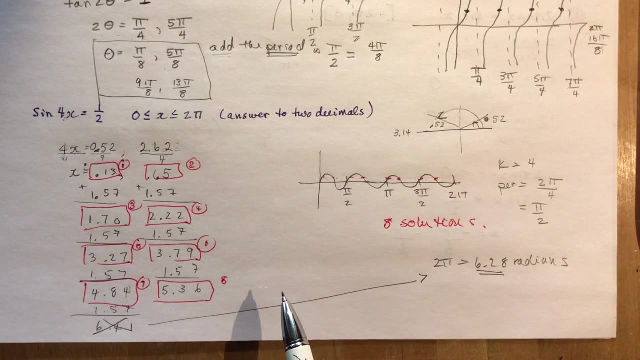 Be careful with these ones where you have a different K value than 1. Because you have to do a little bit of thinking to make sure you're covering all the solutions. Okay, I hope that helped you. It's a snowy day here today. 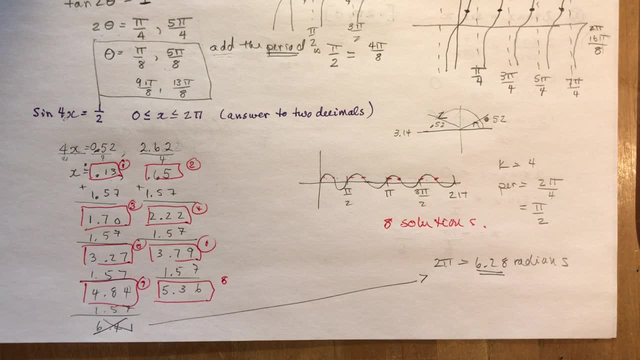 And, like I said, I've got a bit of a cold. Hopefully I'll be able to keep taping for you. Have a great day, Good luck, Bye, bye. 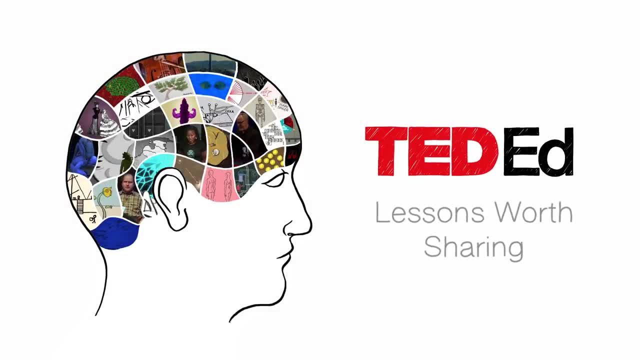 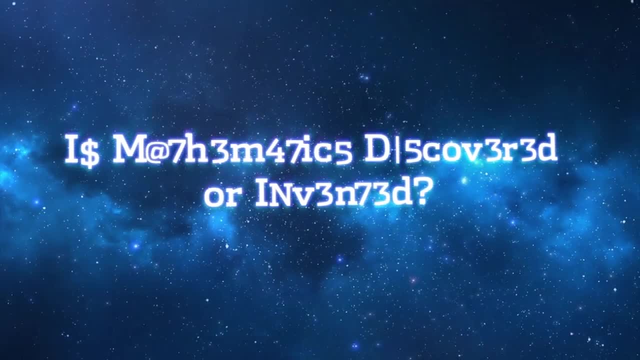 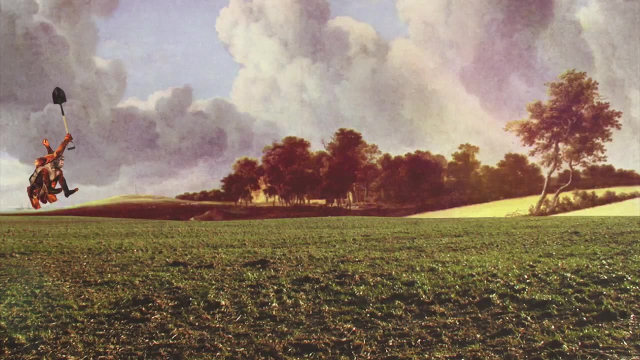 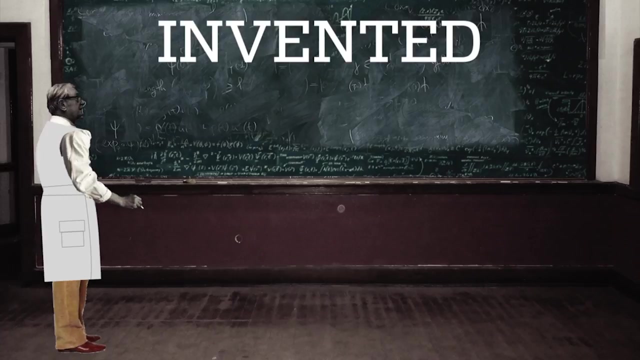 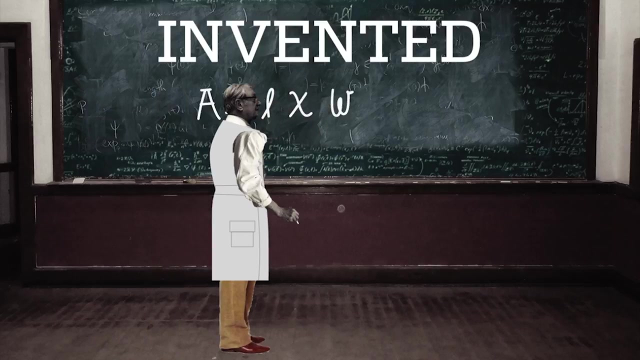 Would mathematics exist if people didn't? Since ancient times, mankind has hotly debated whether mathematics was discovered or invented. Did we create mathematical concepts to help us understand the universe around us, Or is math the native language of the universe itself existing, whether we find its truths or not? 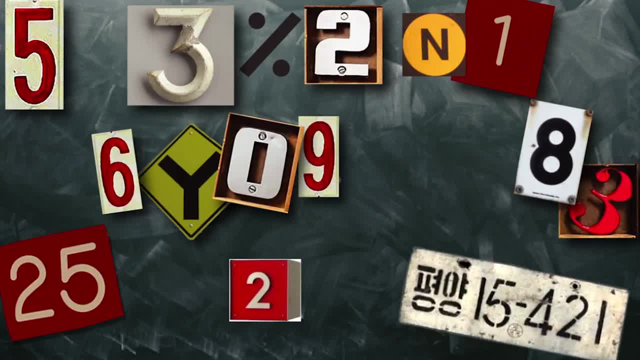 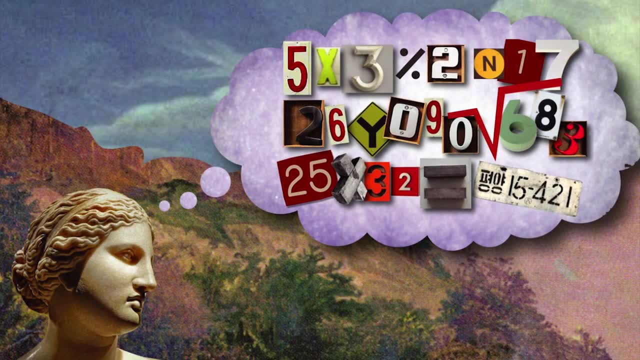 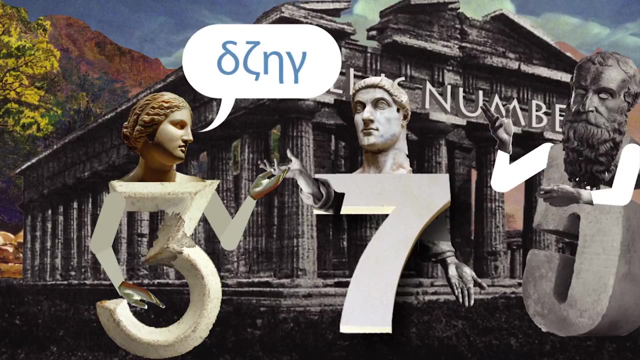 Are numbers, polygons and equations truly real or merely ethereal representations of some theoretical ideal? The independent reality of math has some ancient advocates. The Pythagoreans of 5th century Greece believed numbers were both living entities and universal principles. 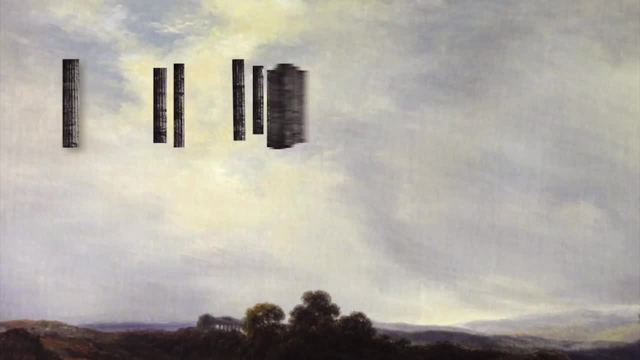 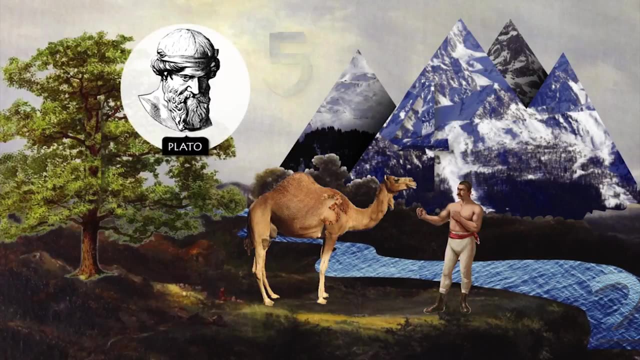 They called the number one, the monad, the generator of all other numbers and source of all creation. Numbers were active agents in nature. Plato argued mathematical concepts were concrete and as real as the universe itself, regardless of our knowledge of them. Euclid, the father of geometry. 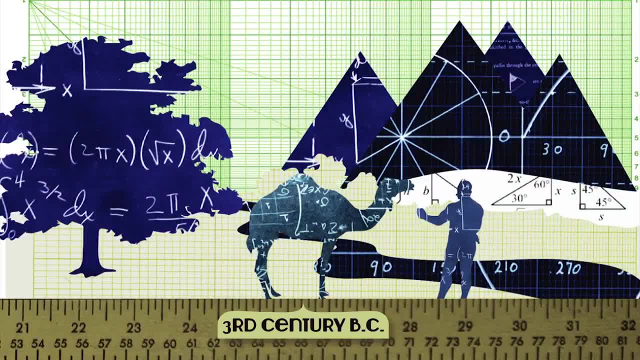 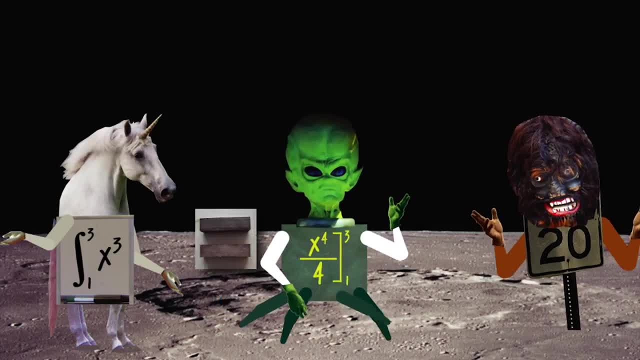 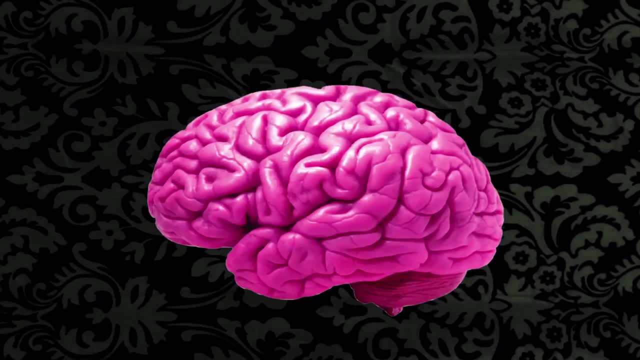 believed nature itself was the physical manifestation of mathematical laws. Others argue that, while numbers may or may not exist physically, mathematical statements definitely don't. Their truth values are based on rules that humans created. Mathematics is thus an invented logic exercise with no existence outside mankind's conscious thought.